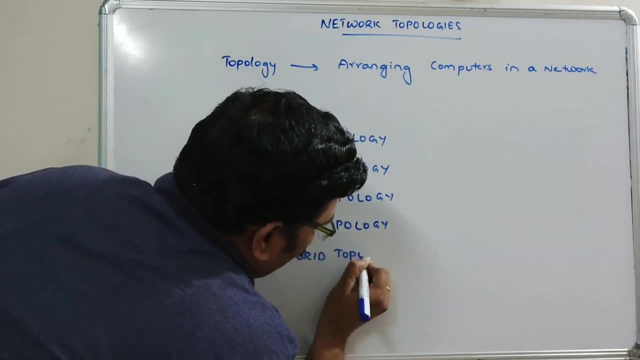 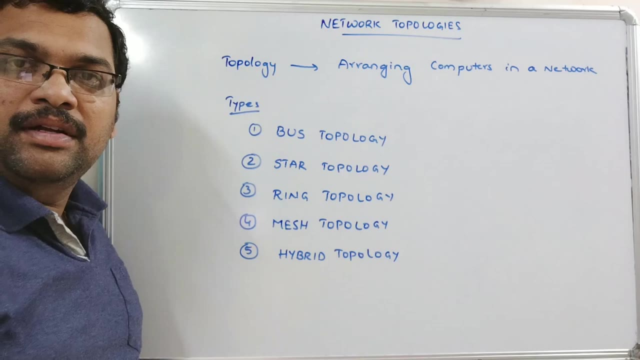 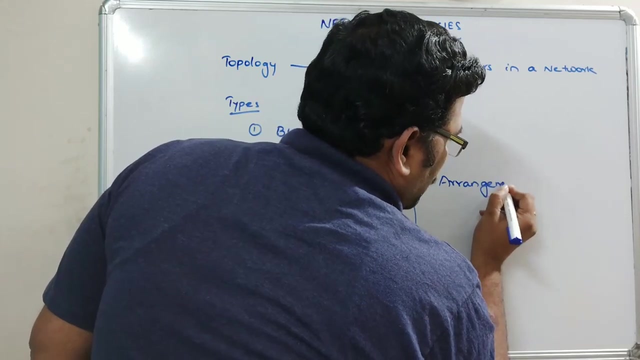 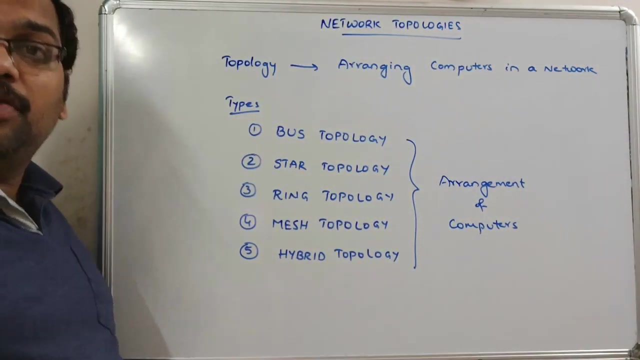 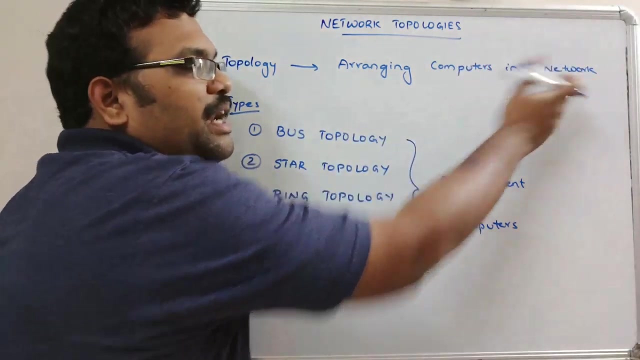 discuss today. So let's get started. So these are the different types of network topologies. so the difference among all these things is arrangement of the computers. arrangement of computers. that means the common thing is, all in all these topologies will connect the computers in the network topologies. 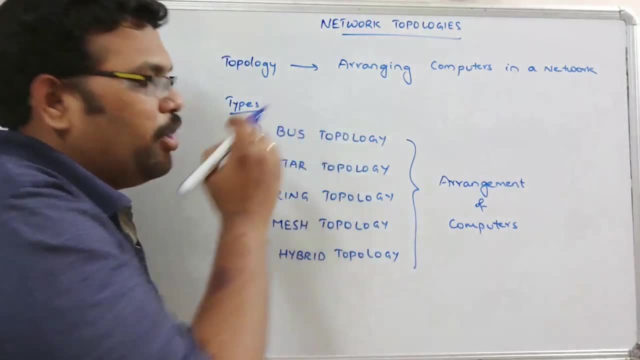 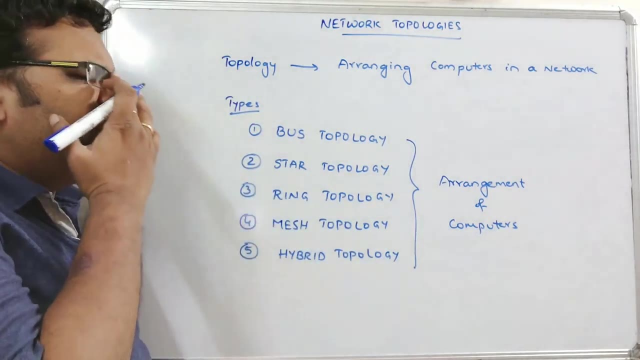 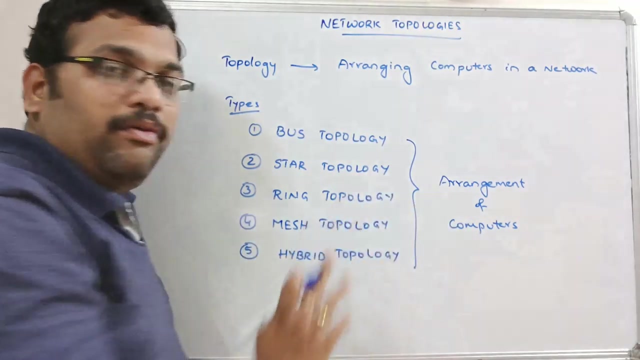 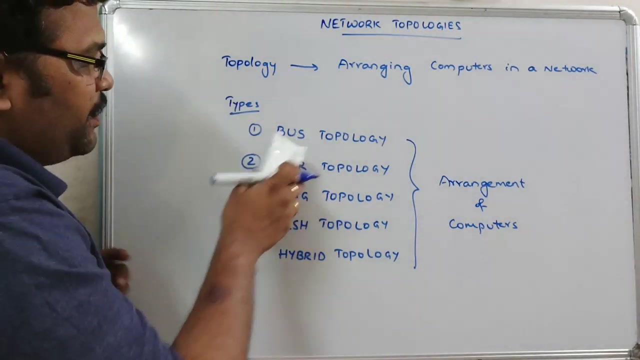 So in all these topologies the data is transferred from one computer to another computer. that means the data sharing is available as well, as the resource sharing will also be available. the only difference is arrangement of computers. so how the computers are being arranged in each topology. now let us see one by one. first consider this bus topology. we will go with. 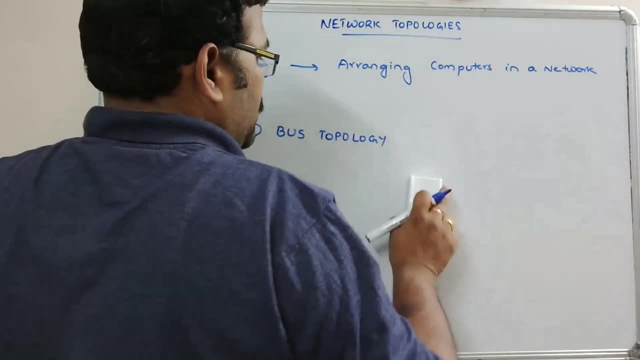 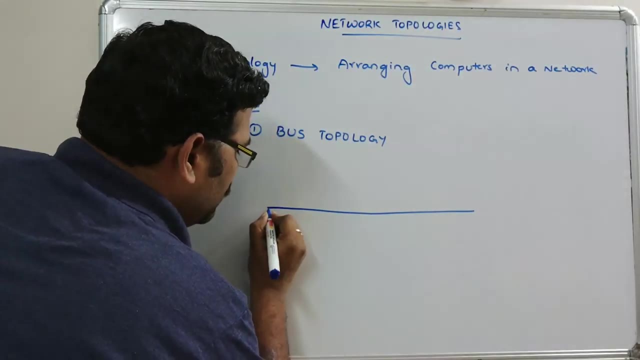 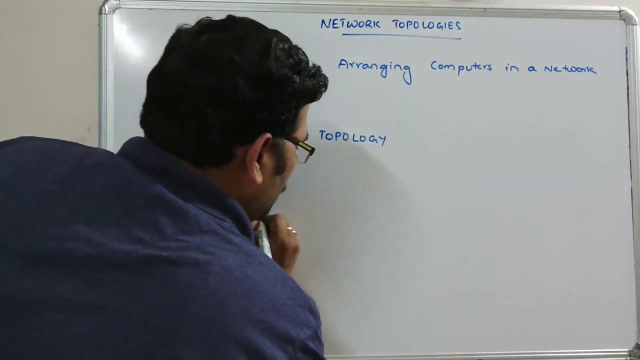 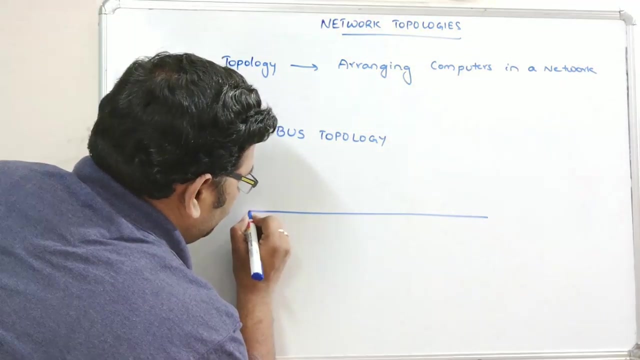 the bus topology. So this is the bus topology. So in this bus topology, so there will be a communication cable. so this is a communication cable, right? so all the computers will be connected only through this cable. See, See, See, See, See. 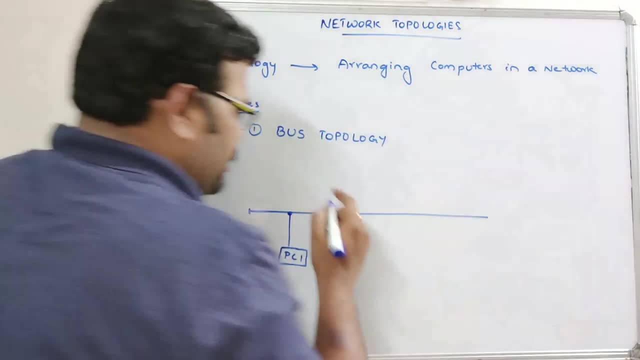 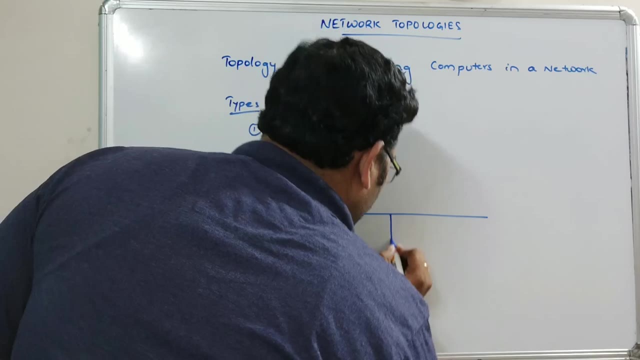 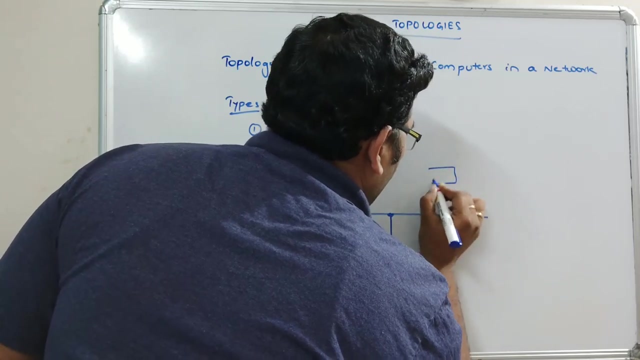 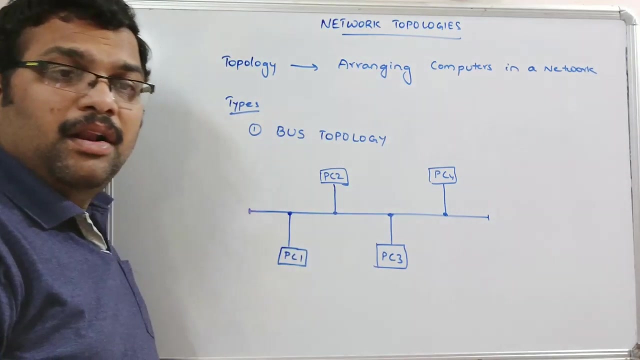 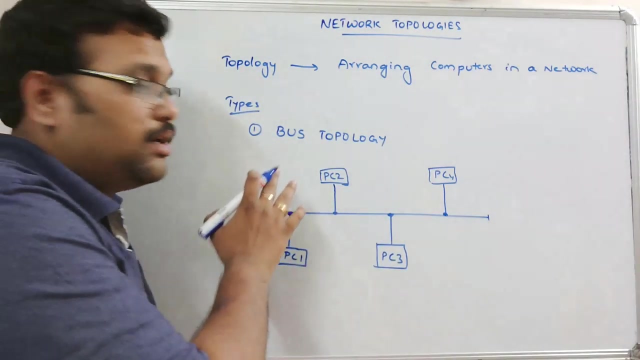 See, See. So this is the bus topology. So personal computer. let us take this PC1, PC2, PC3, PC4, right. So here a small example. we have connected four systems to a single cable, so this is called the bus topology. bus topology, how the i mean this bus is nothing but a line or a cable where the data can be. 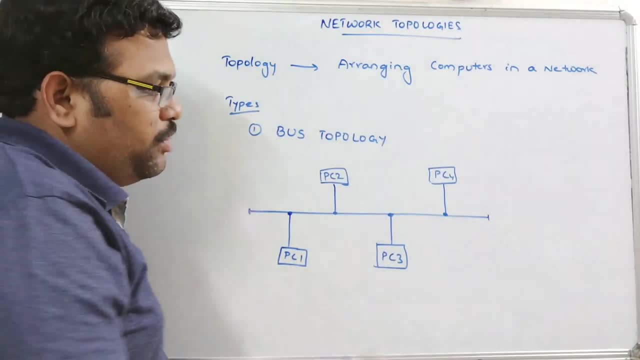 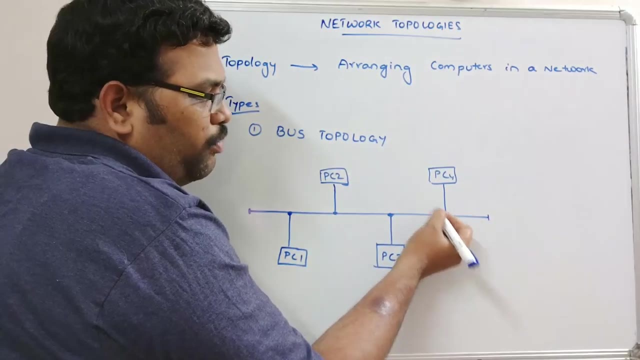 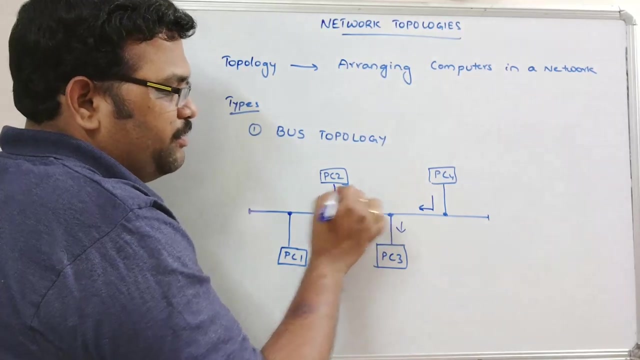 transferred from one system to another system, right, so here, if pc4 wants to communicate with pc2, the data will be moved in this way. okay, so the data will be received here. the data will be received here, right, and also the data will be received here, but based upon the address only. 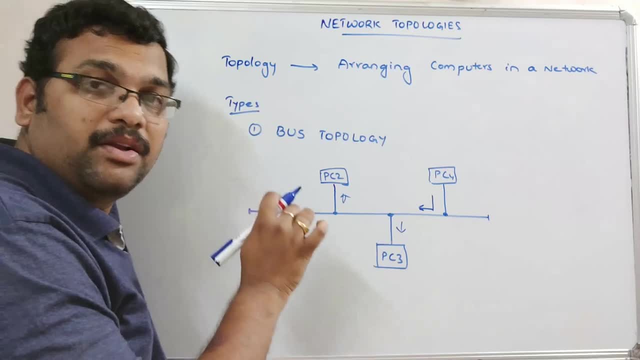 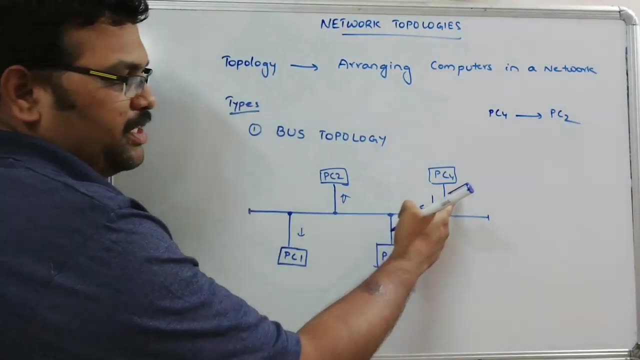 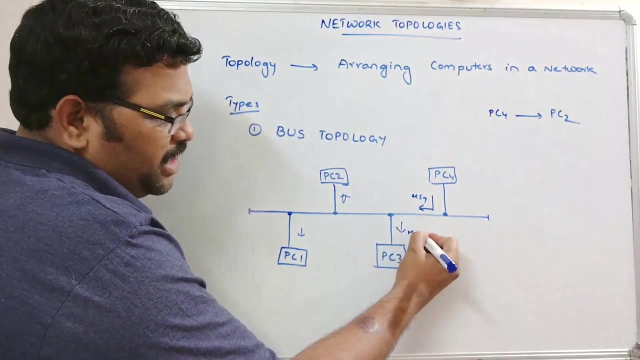 the destination computer will be responding to that particular message. for example, if pc4 wants to communicate with pc2, so pc4 sends the data or a message through this cable. so the same message will be received for pc3 and also the same message will be received for this. 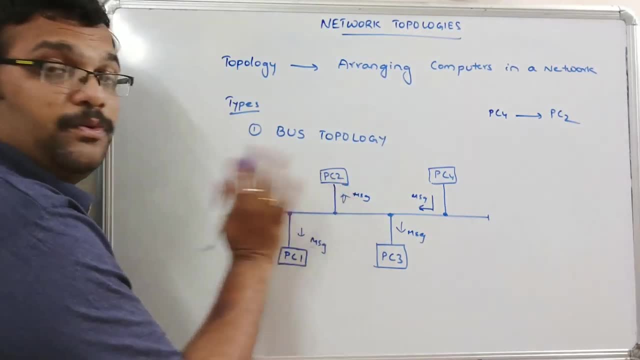 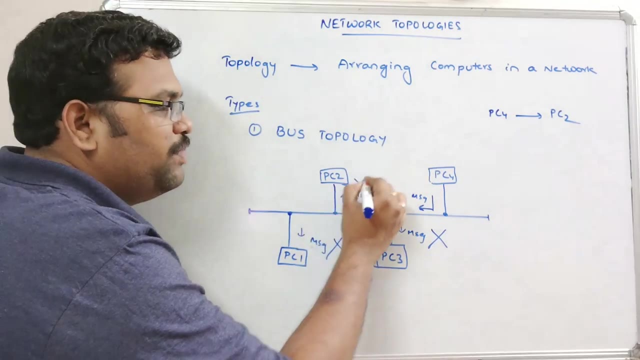 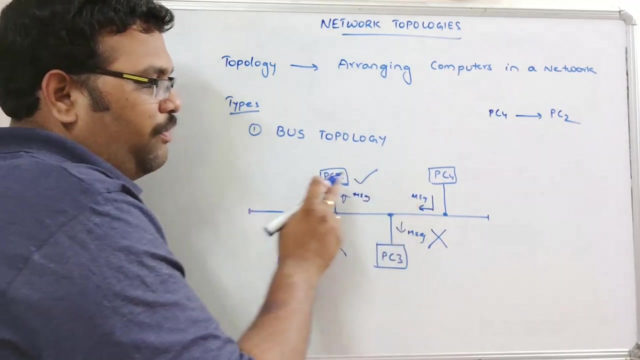 pc1 and pc2 and the same message will be received for this PC2, but PC3 will reject this message. PC1 will reject this message, but PC2 will accept this message, will approve this message. right, because in that message there will be an address of PC2, okay, so this PC2 will respond for that message. 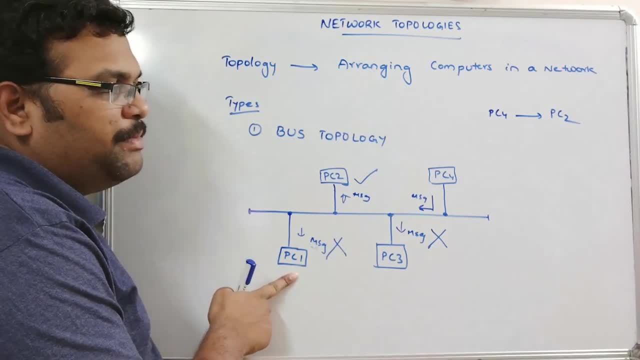 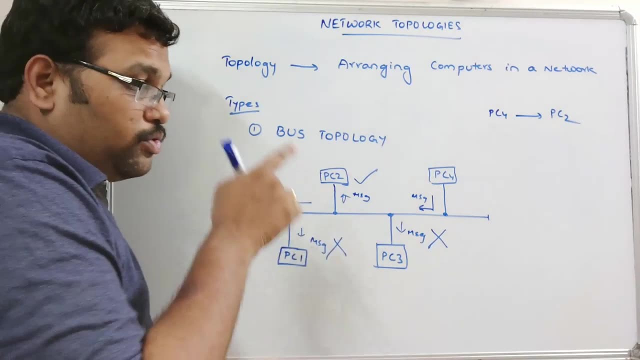 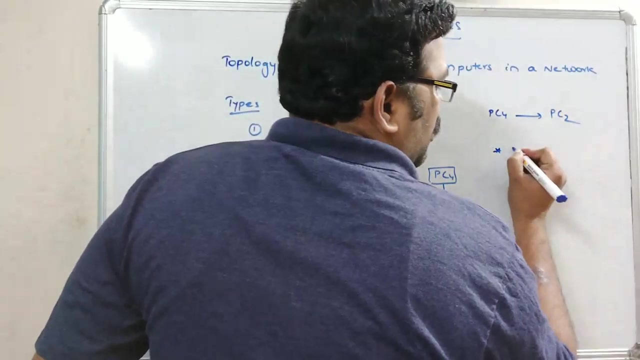 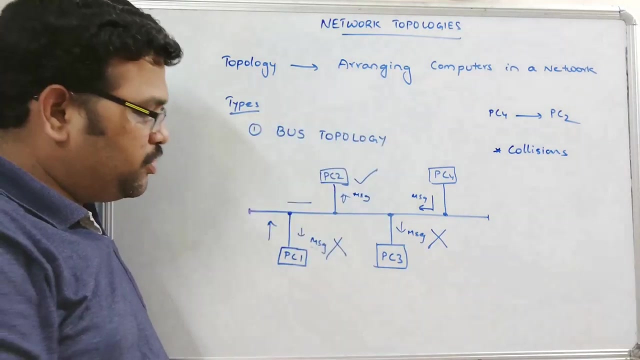 so, similarly, if PC1 wants to send a message to PC4, the message will be sent through this single cable. so hope you understood. so through this single cable the messages will be transferring. so here the main drawback is collisions. there might be a chance of having a data collisions. so if PC1 is sending a message here, similarly PC4 is sending a message here. 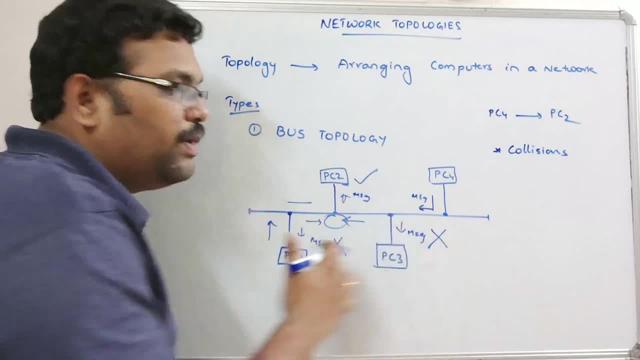 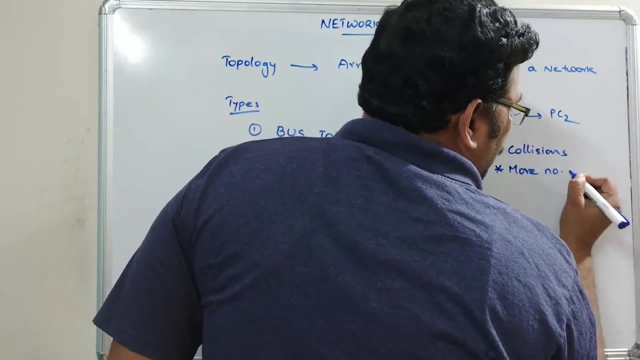 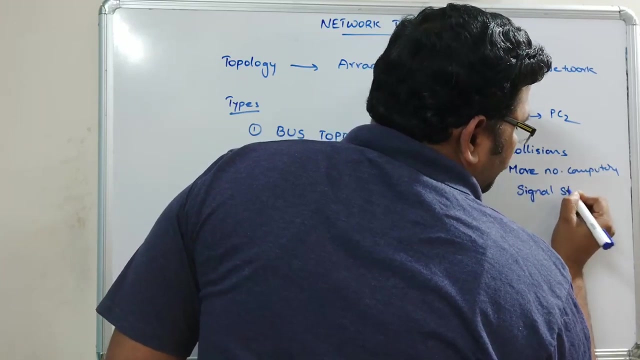 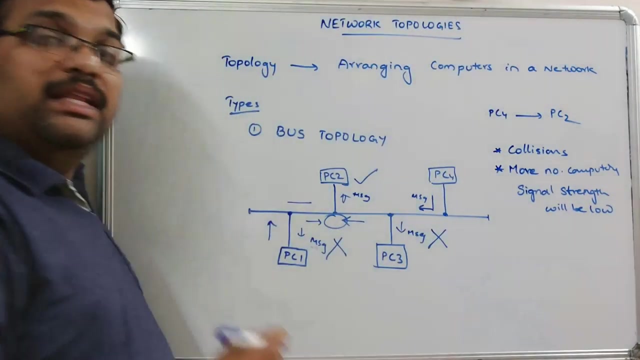 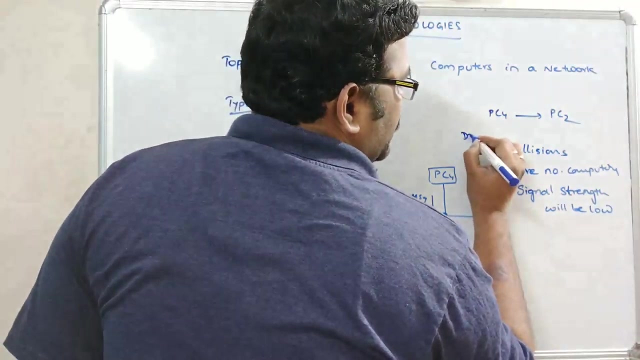 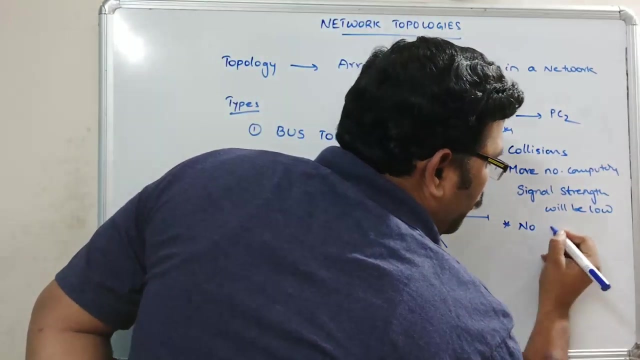 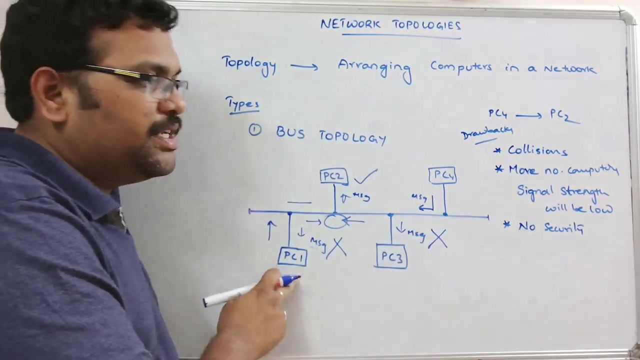 there is a chance of getting collision and this network will be collapsed. and also, if you add more number of computers, signal strength will be low. automatically the signal strength will be decreased. okay, so this is one more drawback. so these are all the drawbacks. and also no security, because every system is receiving the message. every system is receiving the message, so there will be no security for the data transfer. 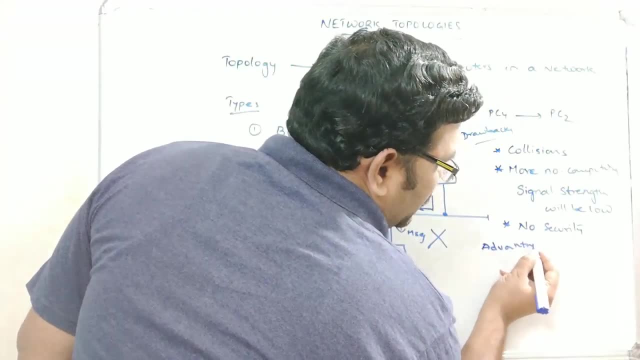 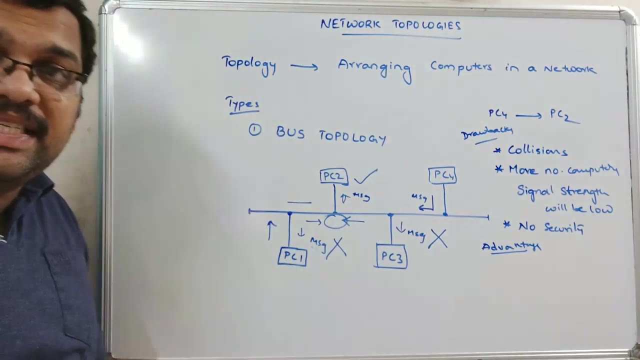 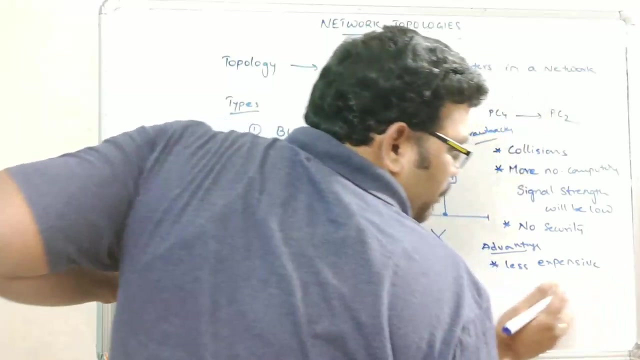 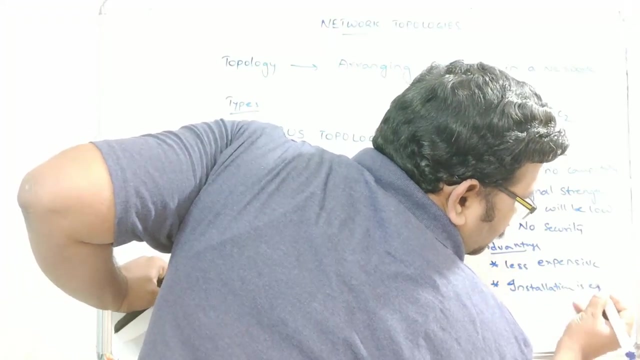 now the advantages. there are few advantages over this bus topology, that is, we are using only one cable, so it is very less expensive to install. less expensive, the cost will be less and installation is easy. right, so we can add more number of computers. 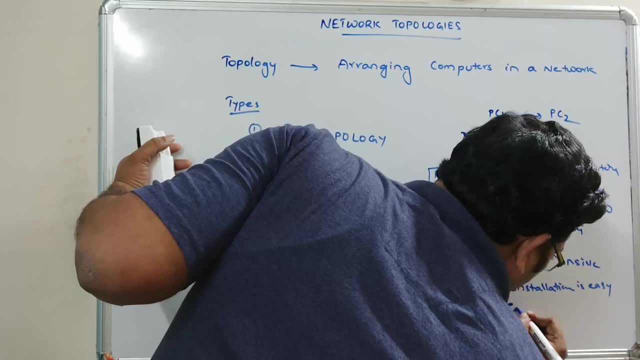 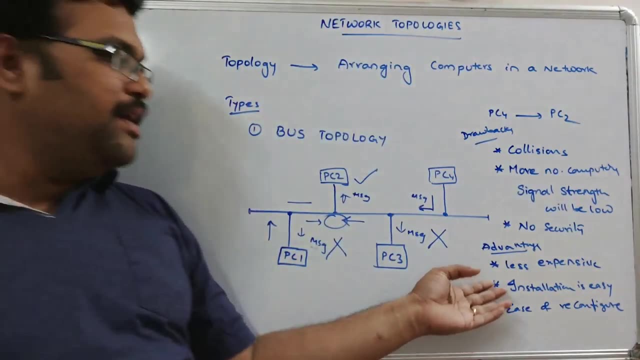 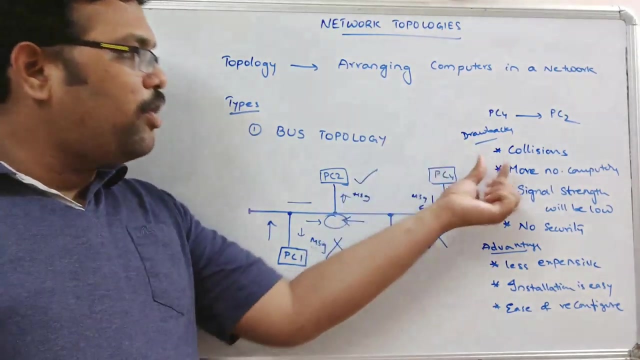 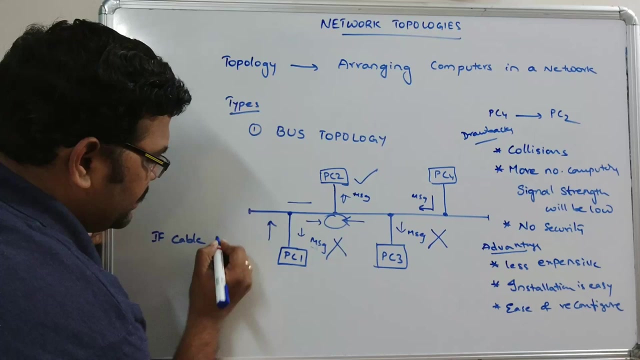 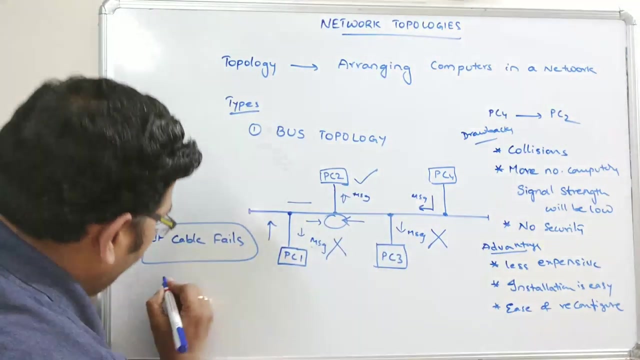 in a simple way: okay, reconfigure, ease of reconfigure, so all these things can be done in this bus topology. so these are some advantages, but there are many drawbacks, because the collision, main drawback- is a collision and also if this cable, if cable fails, if cable fails, the complete network will be collapsed. so 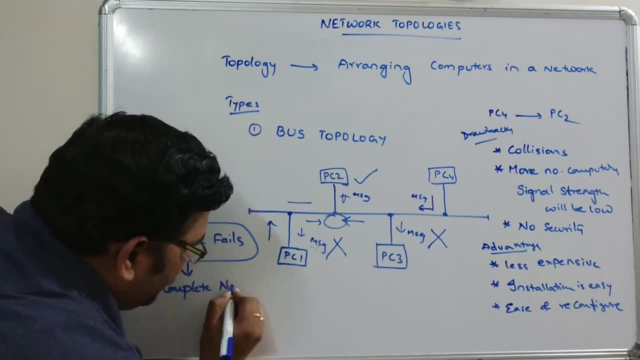 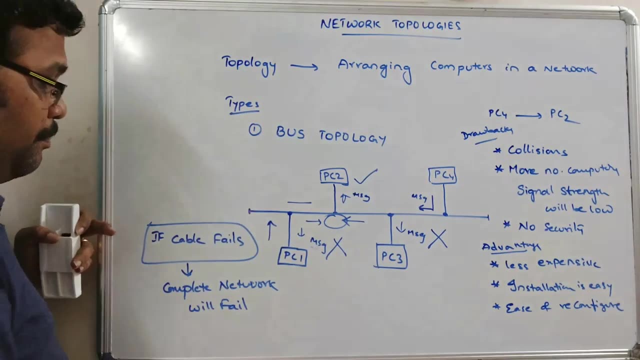 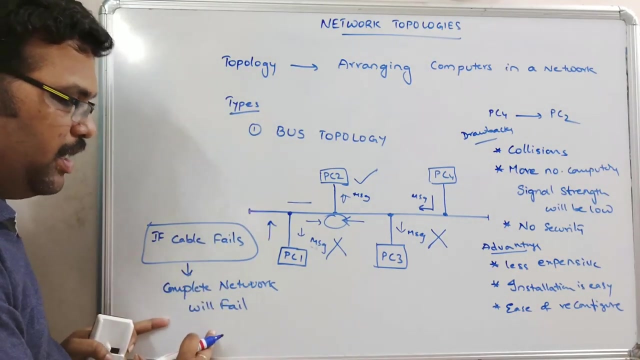 the complete network will be collapsed. so the complete network will be collapsed. it will fail because all the computers are connected to only one cable. so if one, if that cable fails, automatically the complete network will be failed. 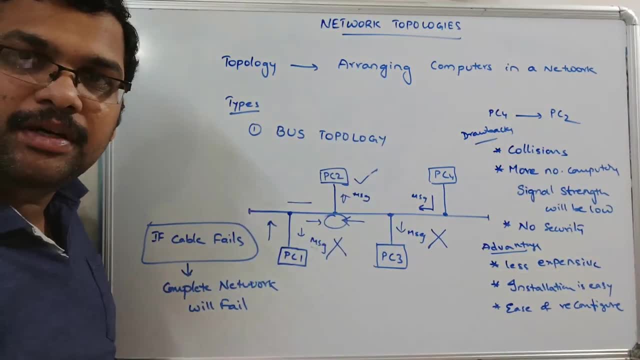 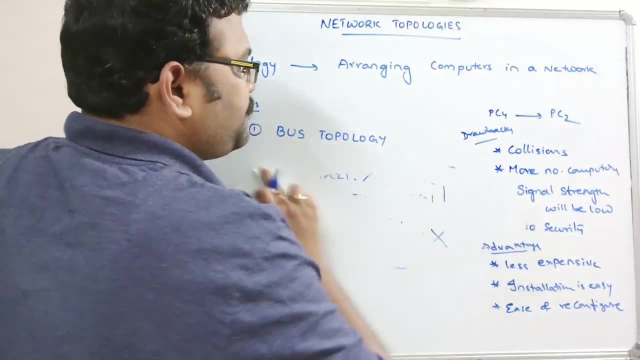 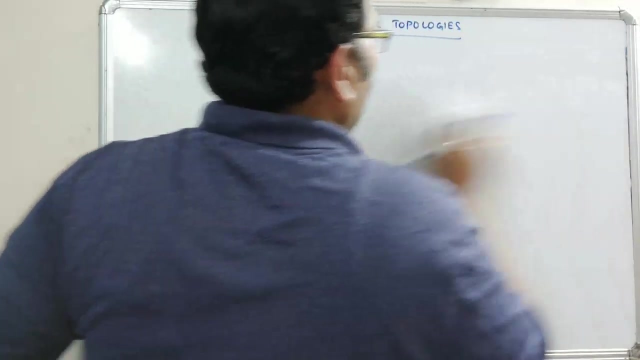 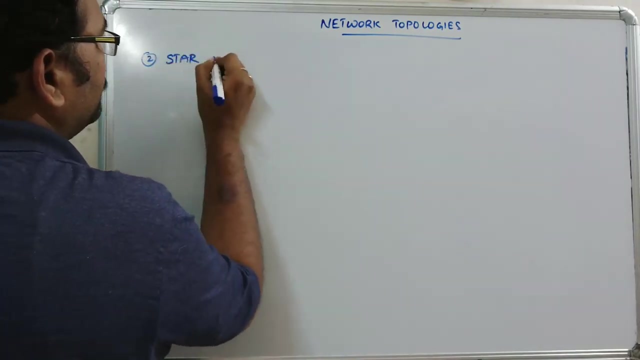 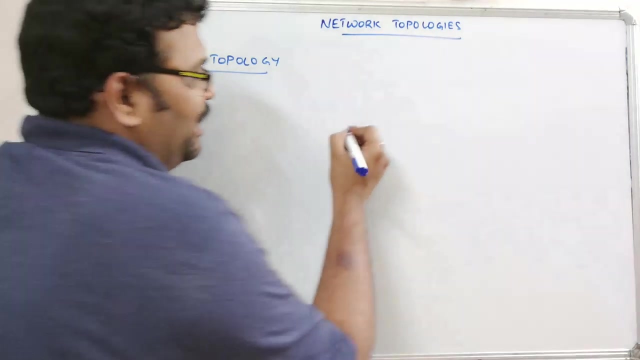 so this is the main drawback of this bus topology: right, so this cable, we call it as a bus. right now we will move on to the next one. the second topology is: this is an automatic change which 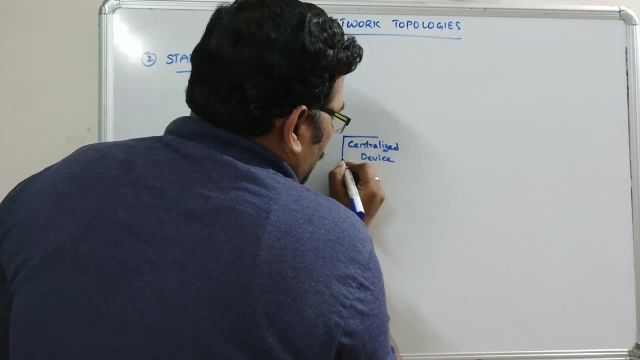 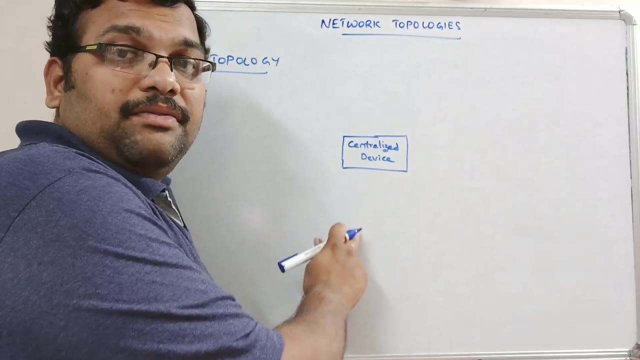 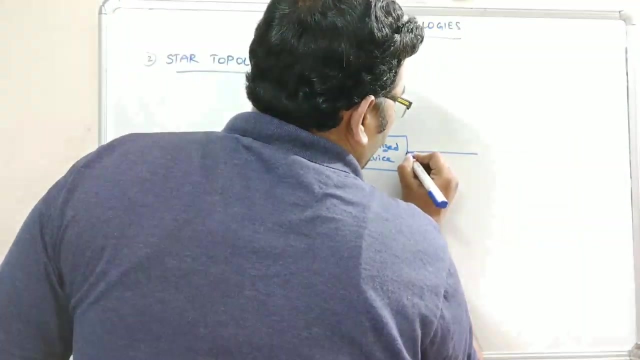 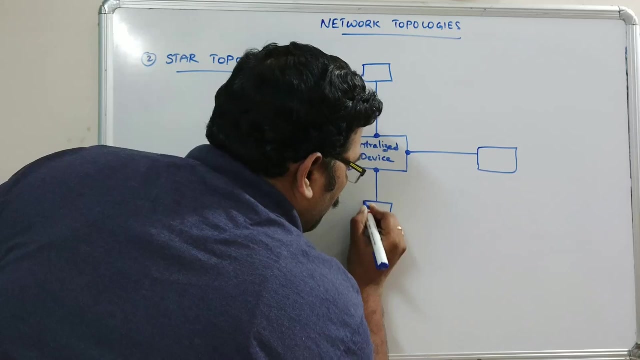 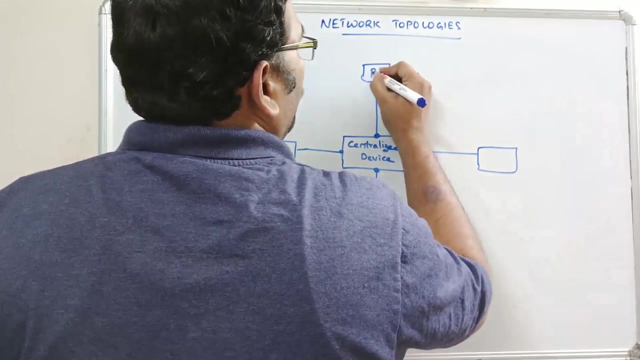 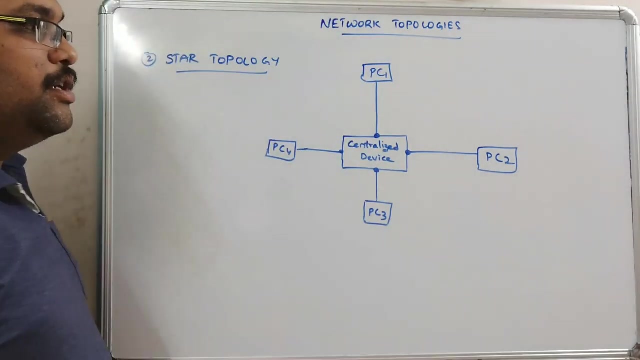 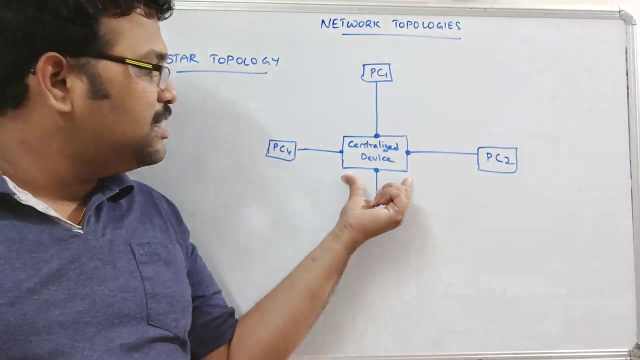 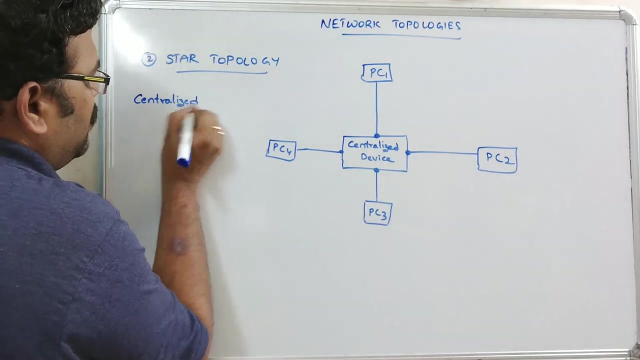 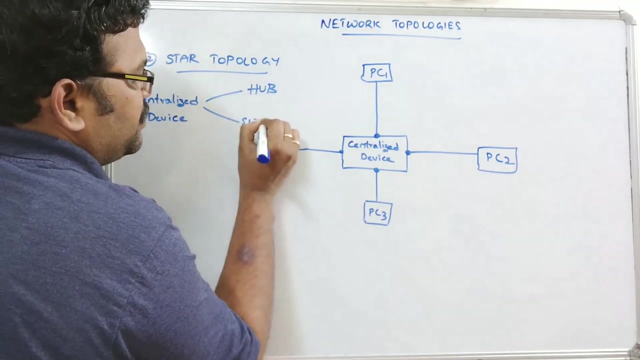 cannot be surprised, because be connected to this centralized device, device. so see, right, so this is a star topology. so all the computers will be connected in a single point to this centralized device. and this centralized device can be either hub or a switch, hub or a switch. so I will tell you the difference between. 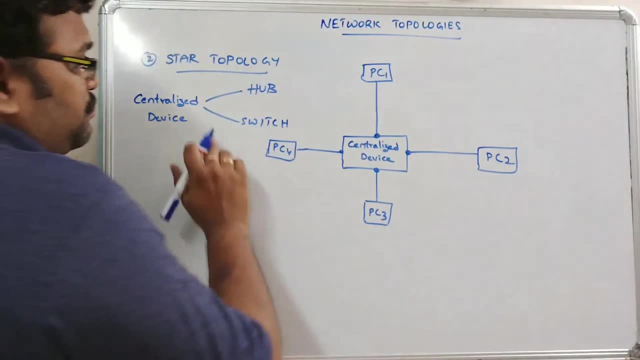 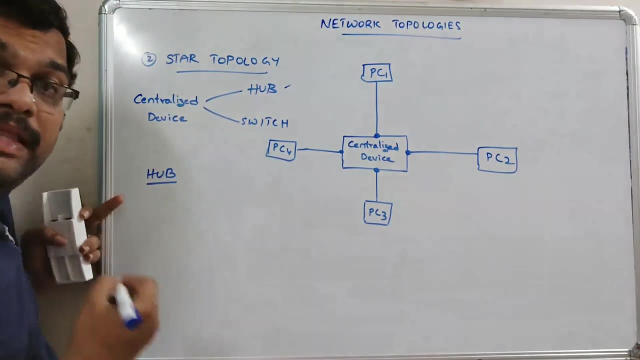 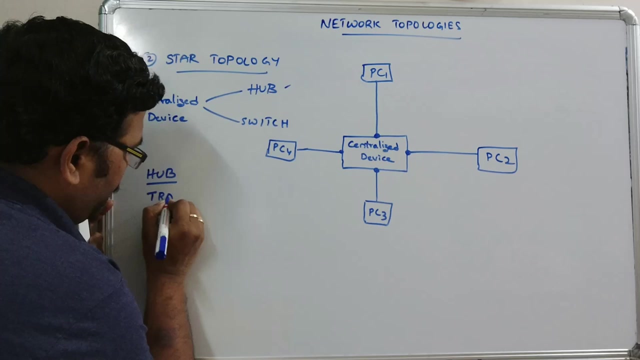 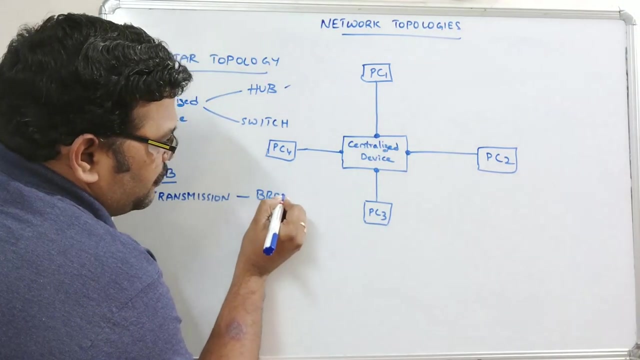 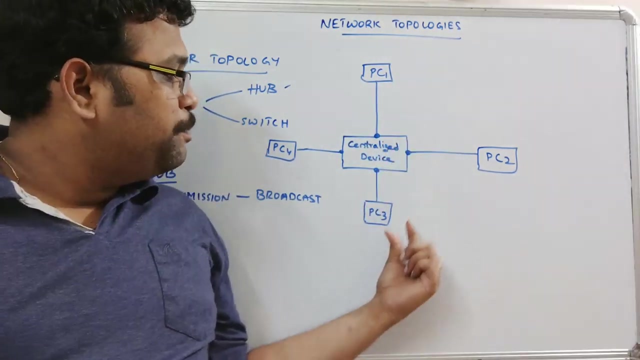 this hub and switch right. so if the centralized device is hub, if the centralized device is hub, then the message transmission will be in a broadcast. transmission will be in a broadcast. broadcast means if PC1 sends the message to PC3, the same message will be transferred to all the computers that are connected in. 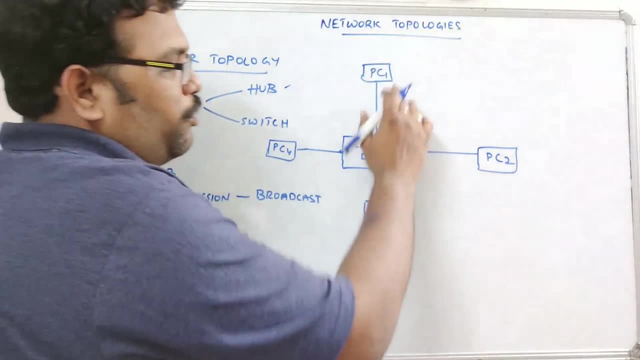 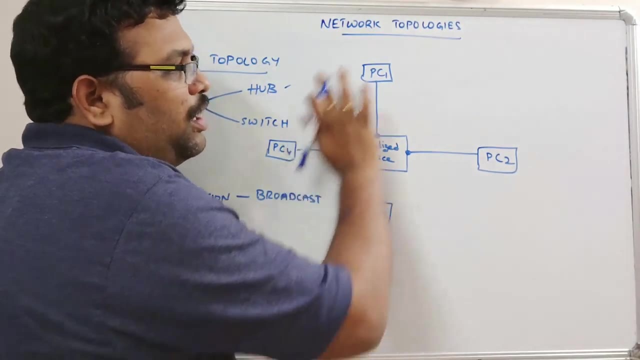 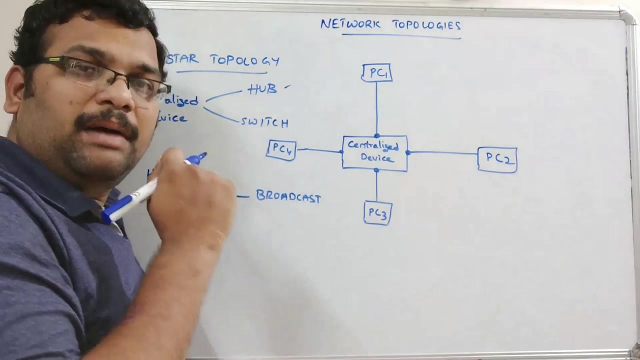 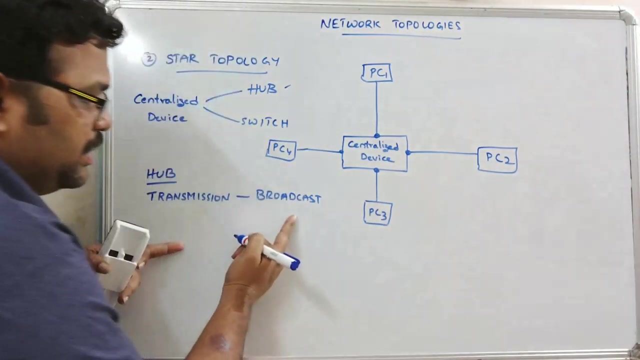 this network. so, first, that message will be routed to this hub and through this hub it will transfer the same message to all the computers which are connected to this network, right? so that is the broadcast, so complete, transferring to all the computers which are connected in the network, right? so this is a 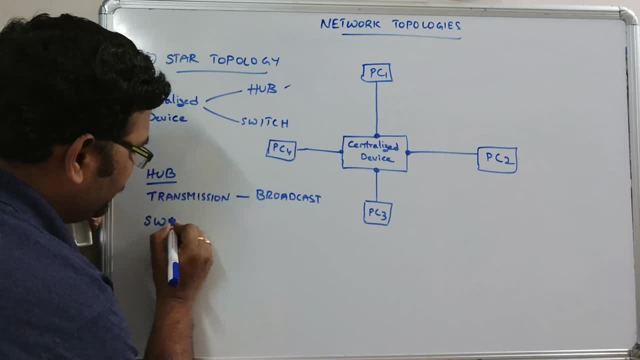 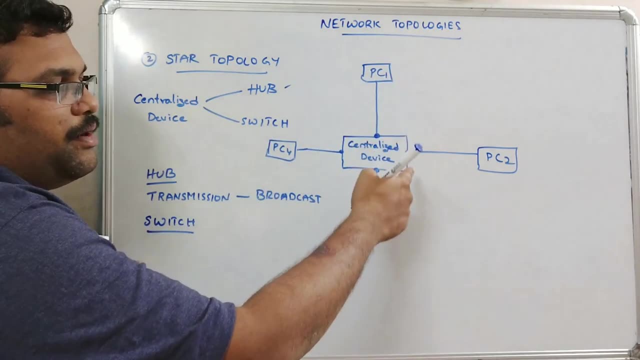 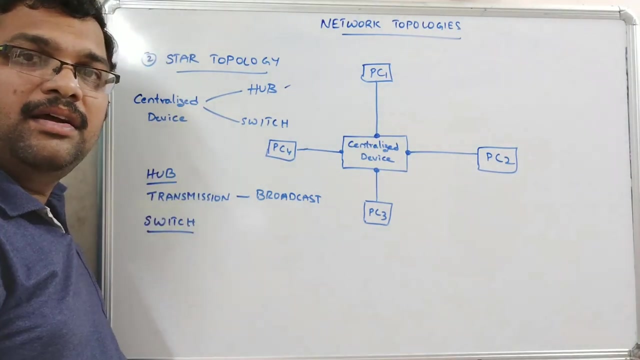 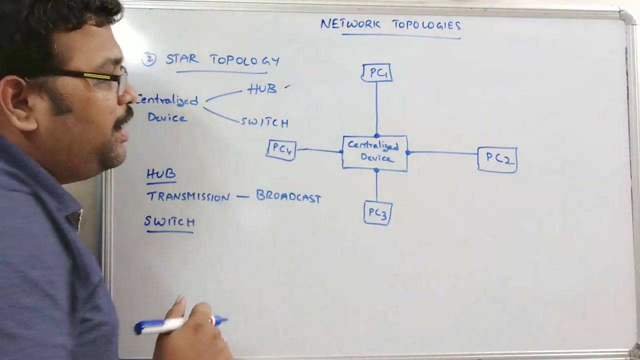 one thing, and if the centralized device is a switch. if the centralized device is a switch, then first the message will be routed to this centralized device so that, based upon the address available in that message, in that message, that message will be transferred to the destination address. right? so see if PC1. 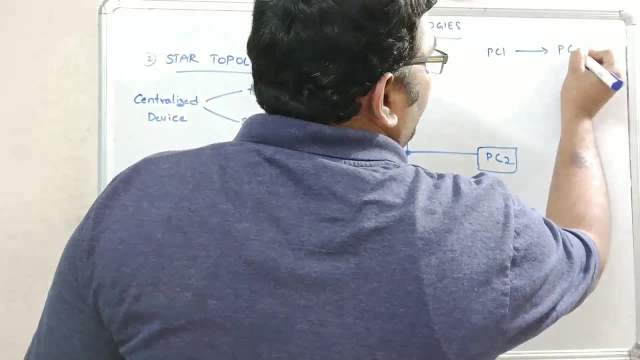 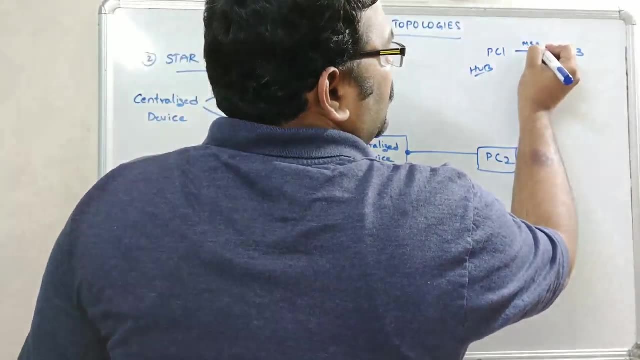 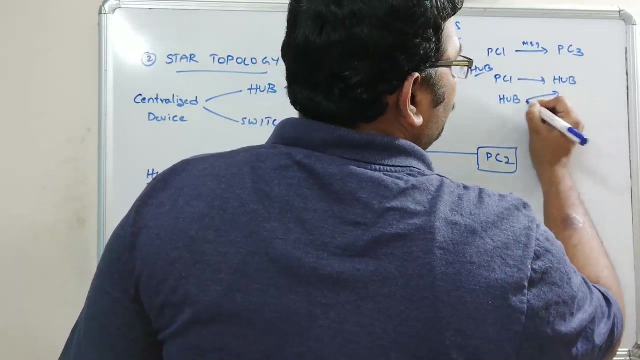 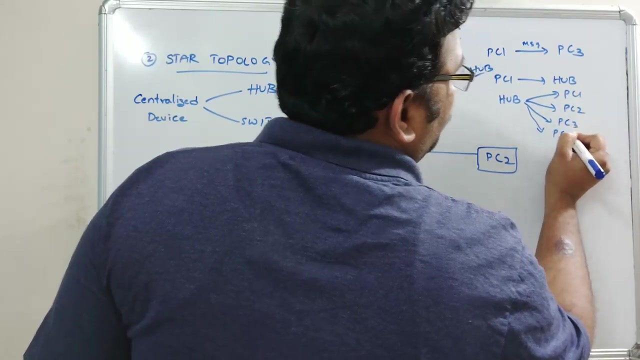 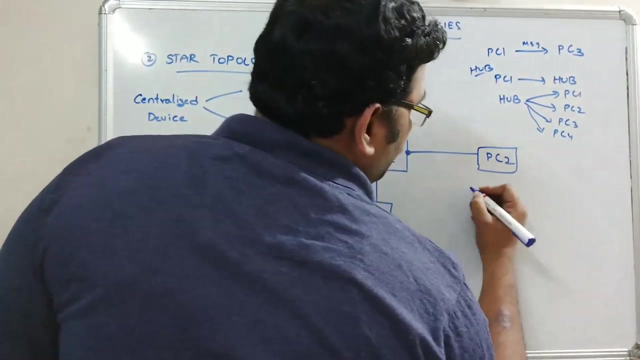 wants to send a message to PC3. three, right, so in hub, if hub is used, right, so message will be routed to hub and through the hub this message will be routed to every system which are connected to the computer. right so this is one thing. and if the centralized 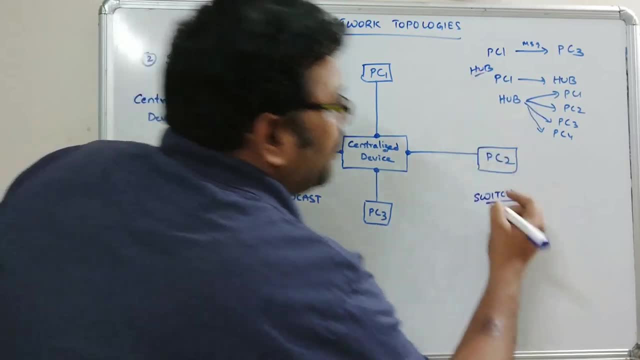 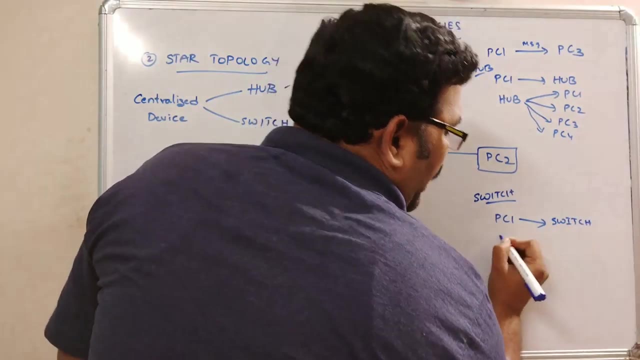 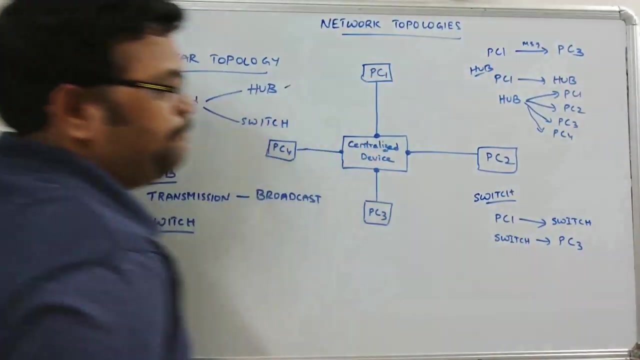 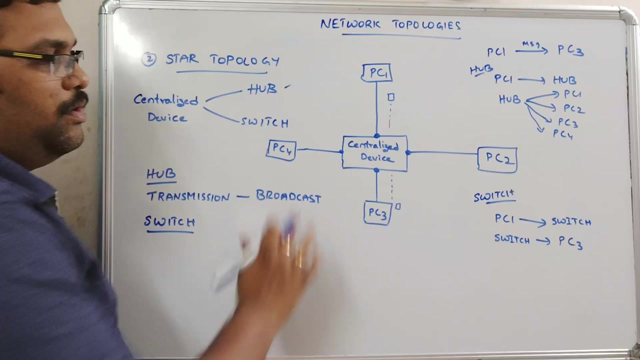 device is switch, then first PC1, the message will be transferred to switch and from the switch the message will be transferred to directly PC3. so a message will be sent from here to here and here to here, so no other system will be receiving this message. so this is the main advantage of using switch right. so multi way connection is. 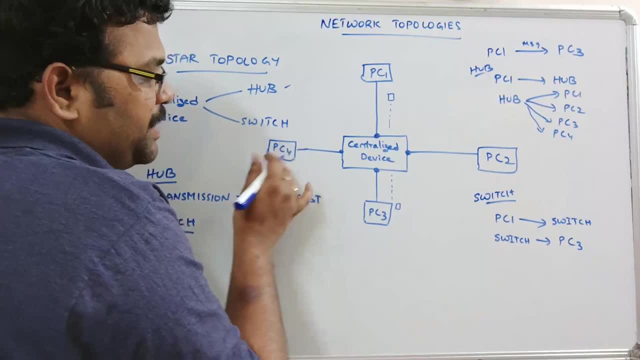 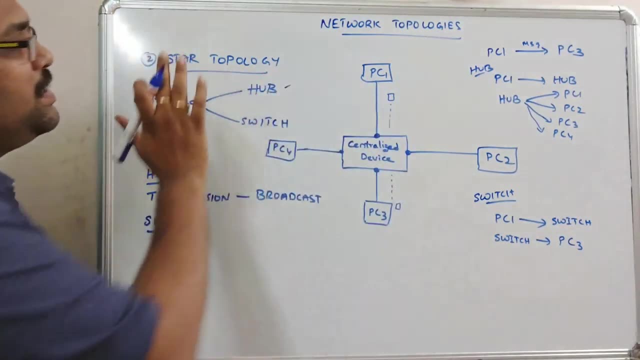 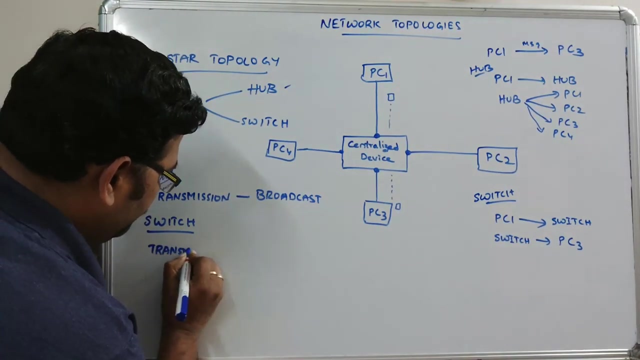 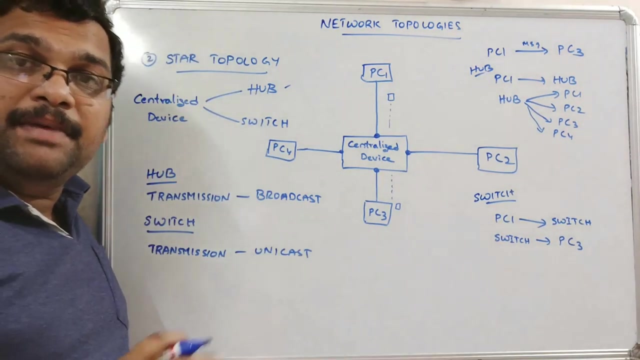 also available. so multiple, I mean so in between- the PC4 can communicate with PC2 also. multi communication is also available. it is also possible in this star topology. so here that transmission, we call it as unicast. unicast means sending the message to only one computer, based upon the destination. 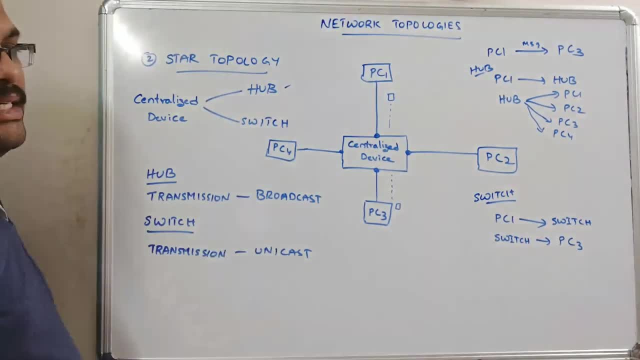 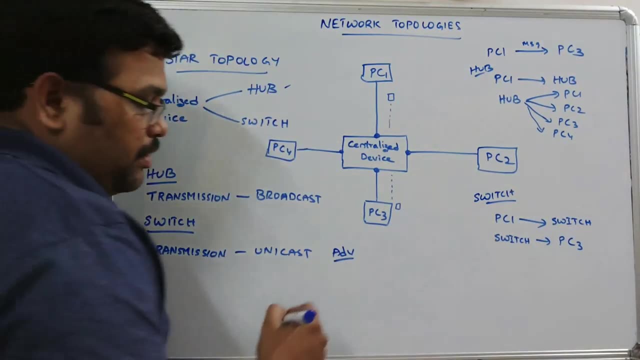 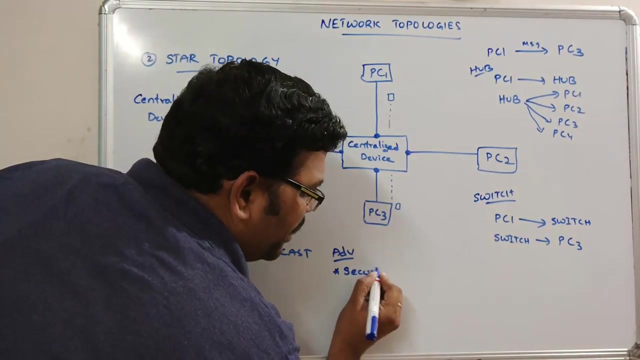 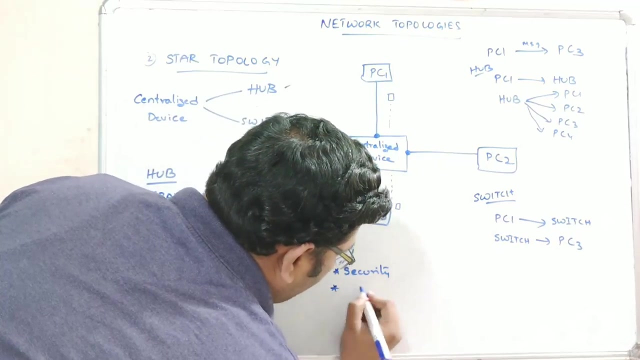 address right. so broadcast and unicast. now advantages, advantages. so if we are using switch, there will be somewhat security. if it is a switch, okay, if the centralized device is a switch, and if it is a switch then it is an unicast, then it is the voice, haha and unicast. 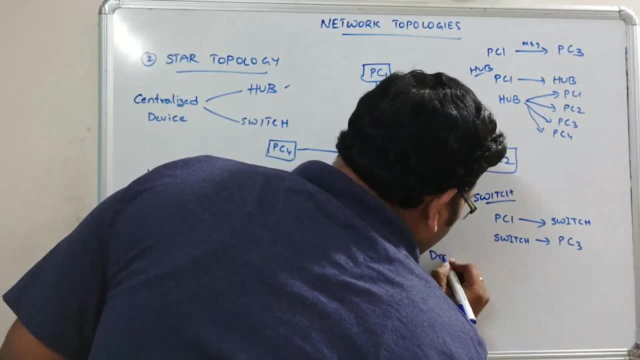 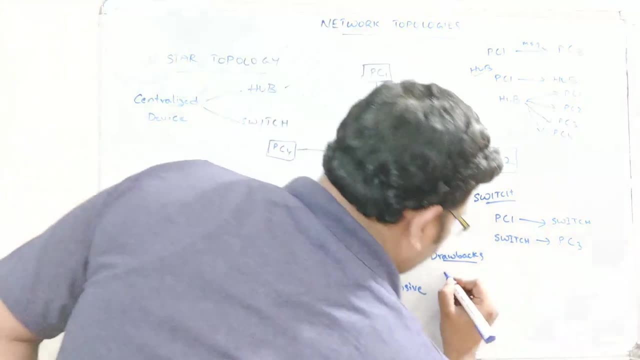 means in this way the device is not connected to the center of the PC1 and the device is working the same way. so that means we are using the same connection, so we have a service in any device. as you can see here, it is fun when we are using the same connection here. on the other hand, it is also 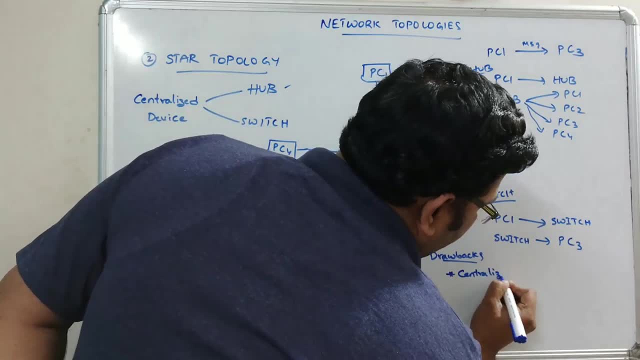 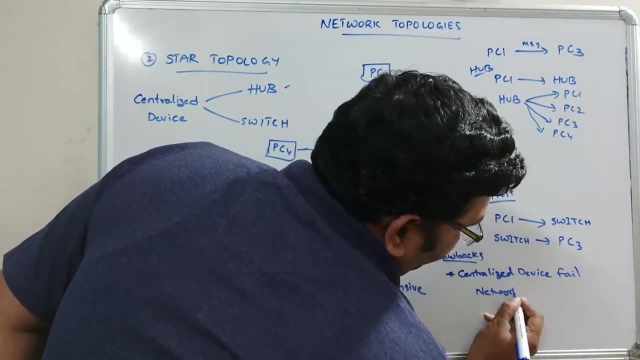 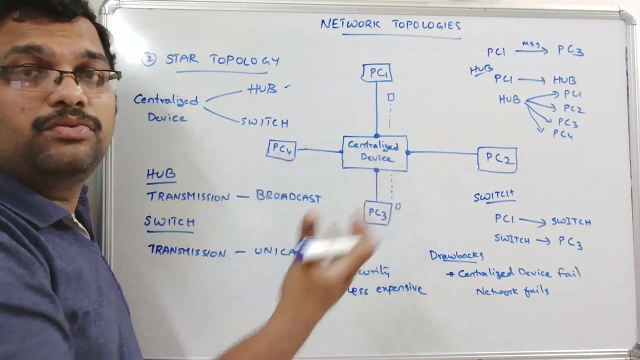 available. so the reason for the reason it is so important is that we are using unicast, because we are using the same connection in this system, so that means there is no need to connect any other things specifically in the similar way. computer- i mean the computers- cannot share the message from one to another, right if this? 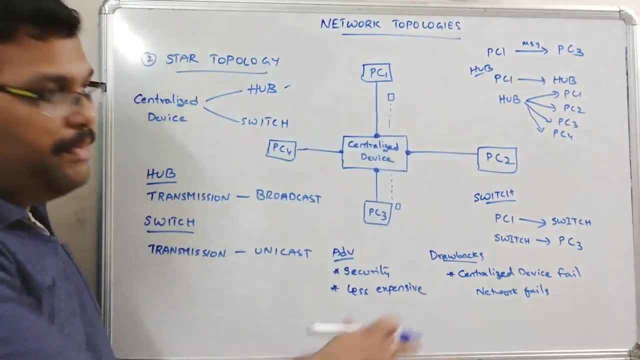 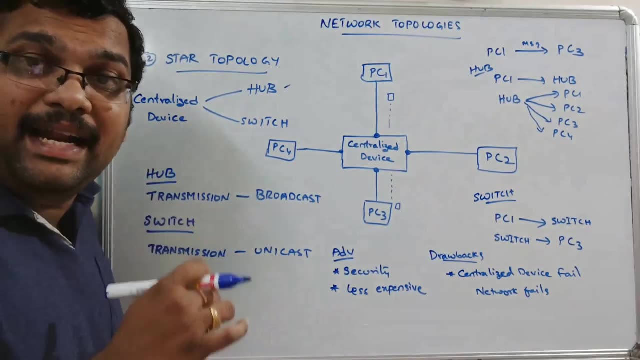 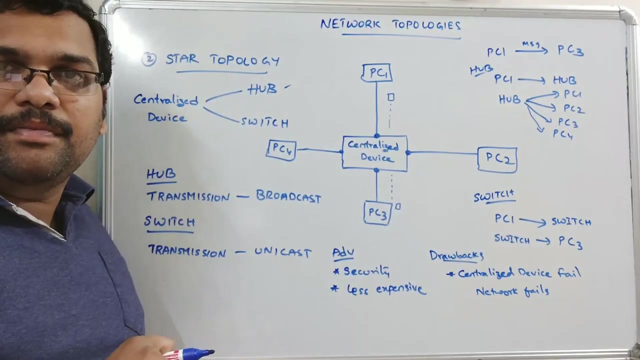 centralized devices fails either hub or switch, there is a main drawback. okay, so this is all about our star topology. so, based upon the address available in that message, that message is routed from the centralized to device to the destination computer. right, so we will go with the next topology. 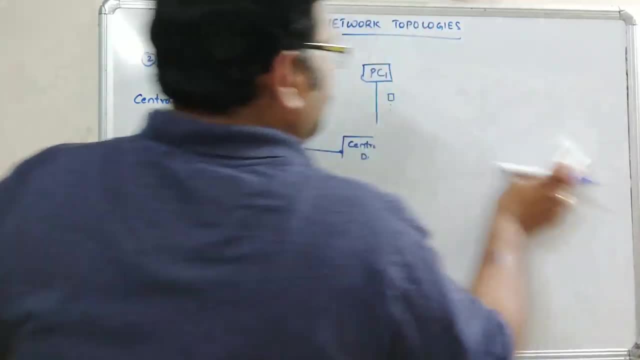 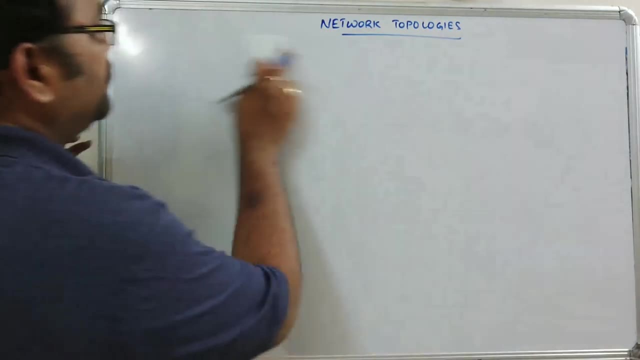 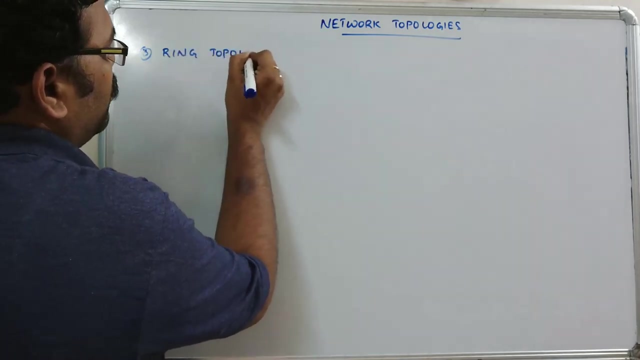 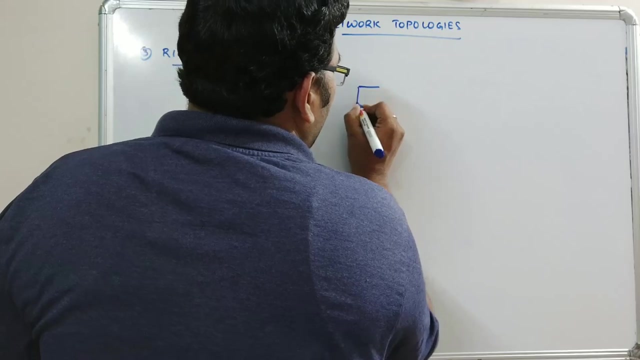 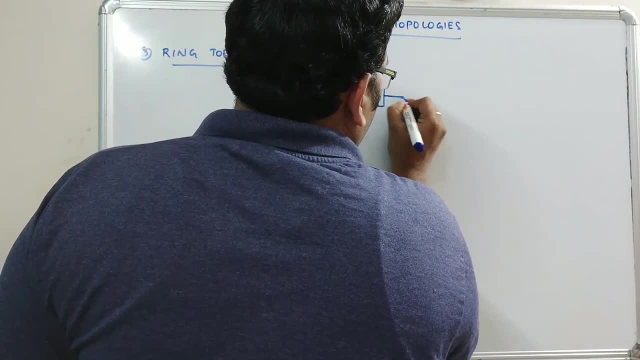 the next topology is ring topology. so in this in topology the systems are connected with the adjacent computers, so see. the next topology is ring topology. so in this in topology the systems are connected with the adjacent computers, so see. so in this in topology the systems are connected with the adjacent computers, so see. 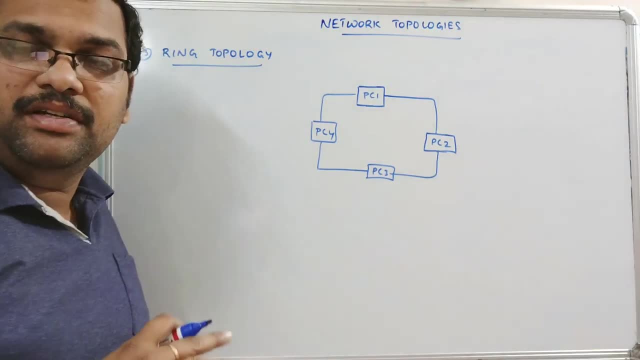 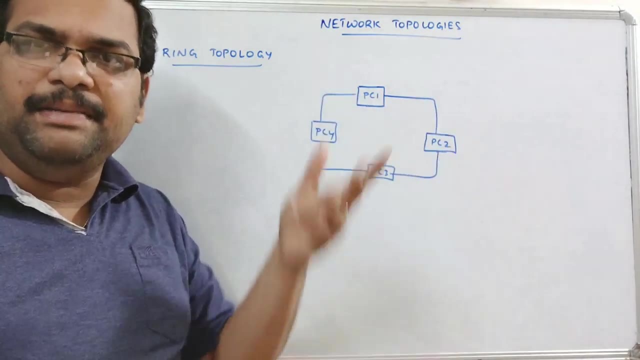 so we got it as a PC1, PC2 or PC3 of nodes. simply, in a network Any computer will be considered as a node, so we can be considered as Node 1, Node 2, Node 3,, Node 4 or PC personal computers. 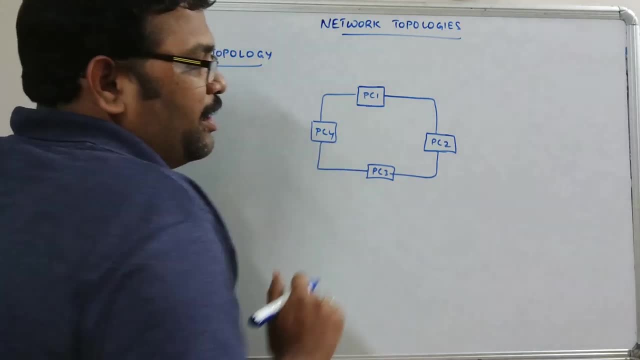 so we can be considered as Node 1,, Node 2,, Node 3,, Node 4 or PC personal computers. so see personal computer 1, 2, 3, 4, right so here. so this is a ring topology so that every computer will. 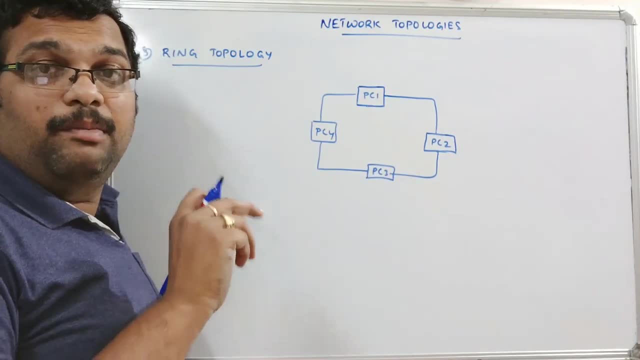 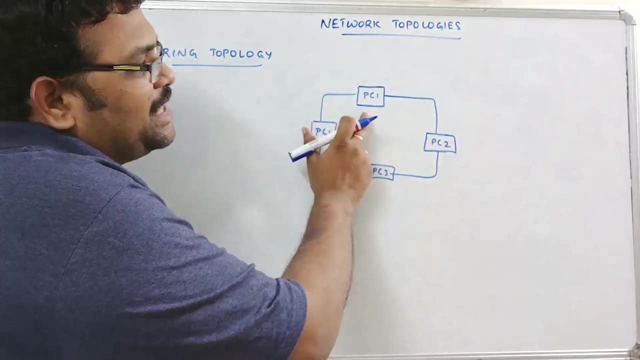 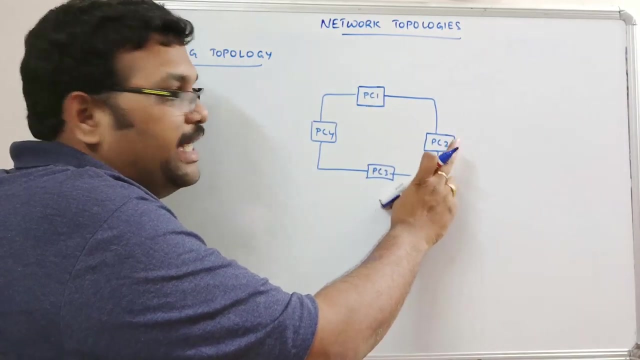 be connected to its adjacent computers. that means it will be having a connection with two computers, one on right side, another one on left side. see, if you consider pc1, it is connected with pc2 and pc4 because these two are the adjacent to pc1. if you consider this, pc2, it 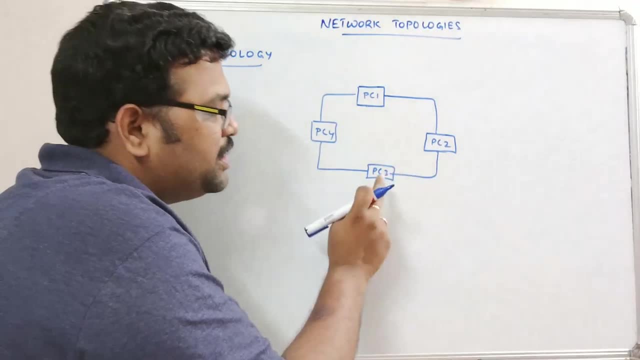 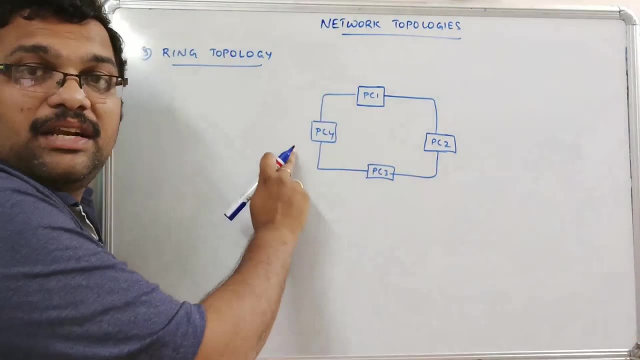 is connected with pc1 and pc3, two adjacents. if you consider pc3, pc4 and pc2, so these two are the adjacents. if you consider pc4, pc1 and pc3, these two are the adjacent of this one. so every computer. 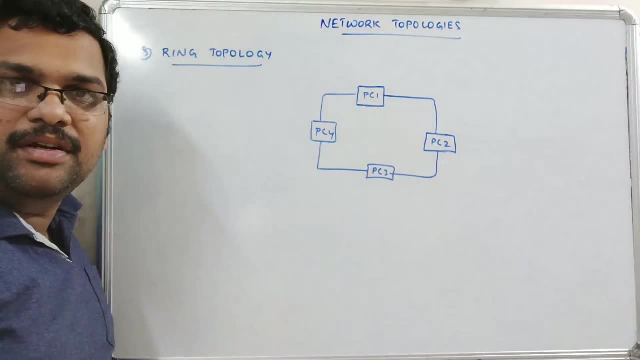 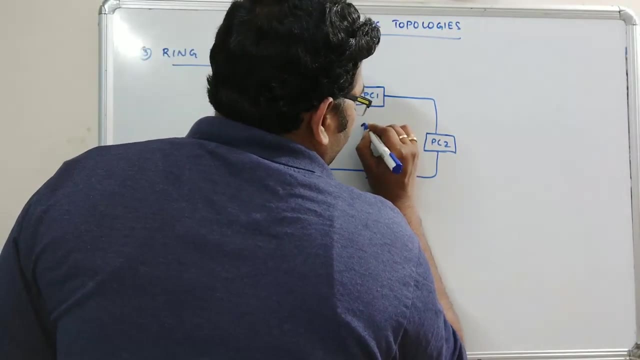 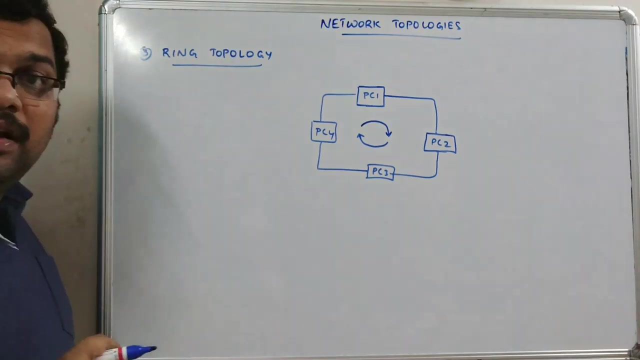 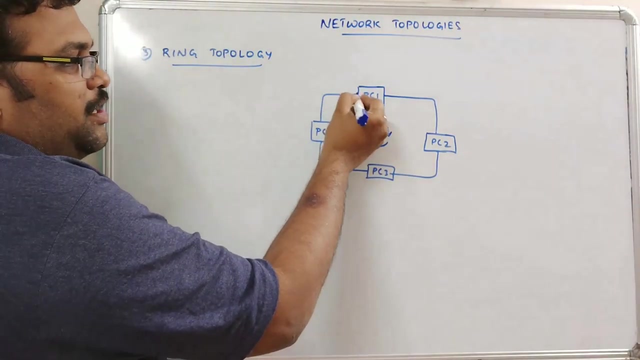 will be connected to its adjacent nodes or adjacent computers. right, so here the data will be transferred in only unidirectional, in a circular fashion. so data is transferred in a unidirectional. so data is transferred in a unidirectional in a circular fashion. so if pc1 wants to send the message to pc4, it's a unidirectional. the message will be sent in this. 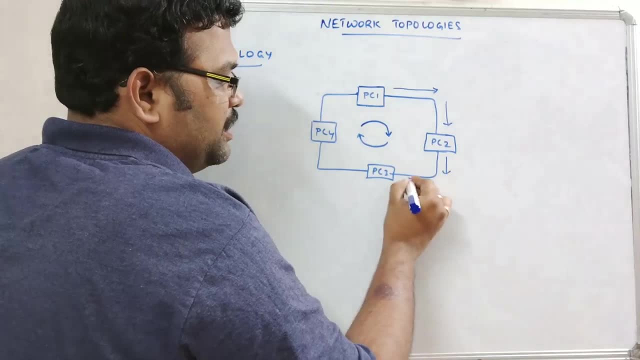 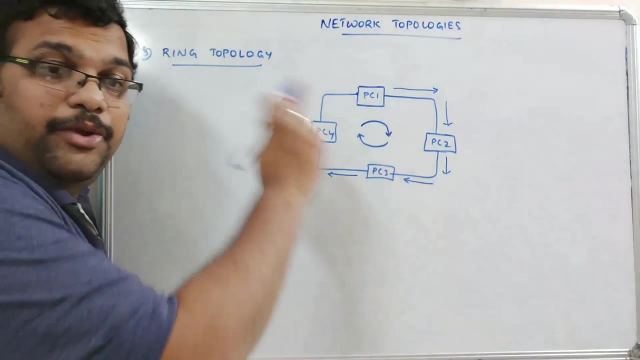 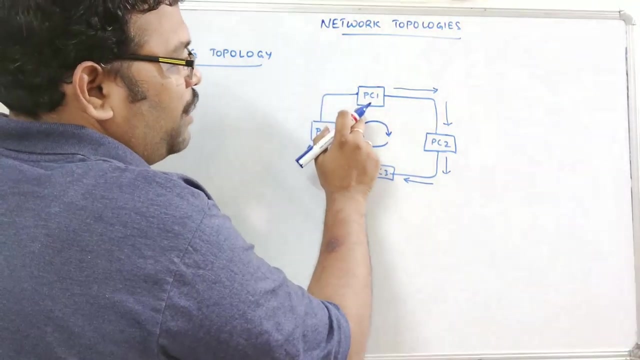 way, in this way, in this way, and finally it reaches to its. this direction, right? so? only unidirectional, in only one direction, right? see, this is the direction of the transmission data. so if pc1, if pc2 wants to send the message to pc3, again the same thing in this directional, in this. 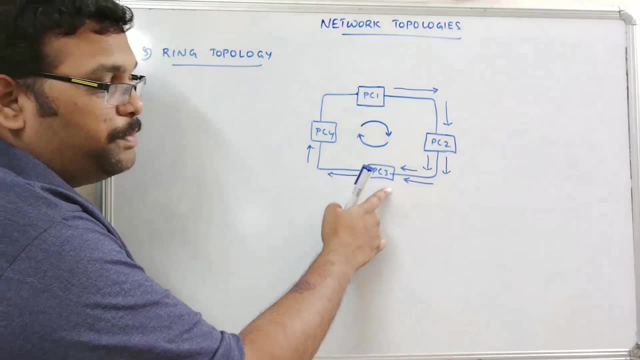 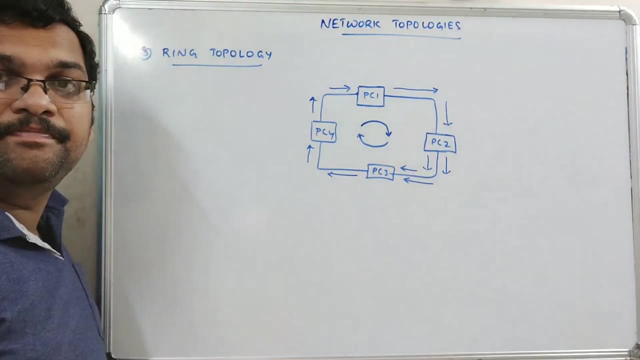 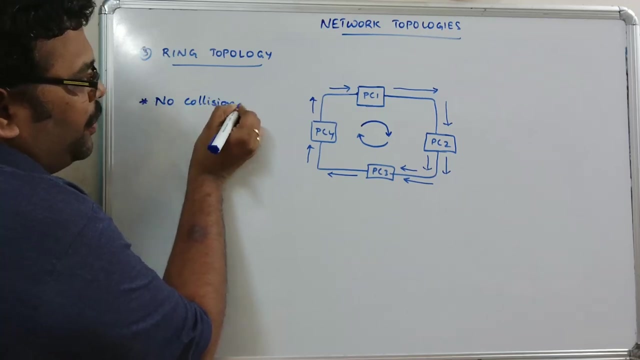 directional and if pc4 wants to send a message to pc3, again only in one direction, right. in this way the data will be sent. so here, no collisions, because the data will be transmitted in only one direction. so there will be no collision, right? so if the data is transmitted in one direction, 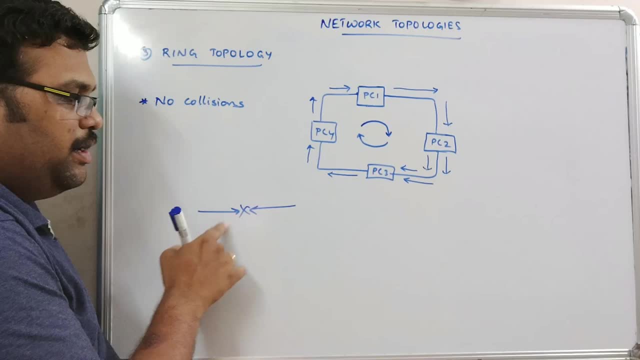 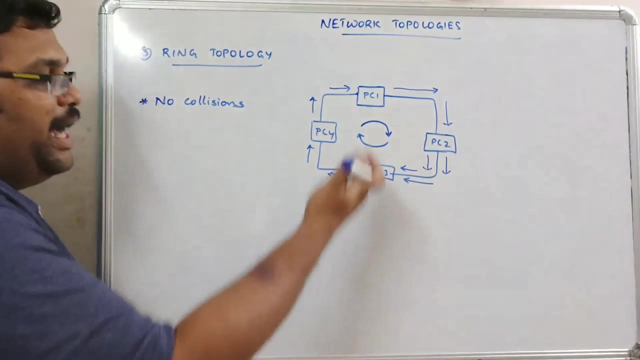 then we call it is a collision, right, if one message is coming from left side and one message is coming from right side, so both will be collided. so this is called a collision, and here there is no chance of getting collision because the data will be transferred in only one direction. that is a 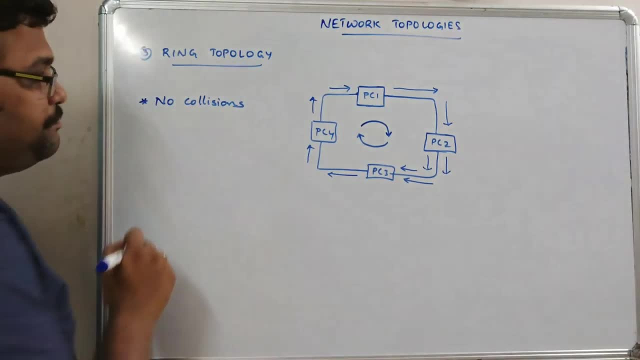 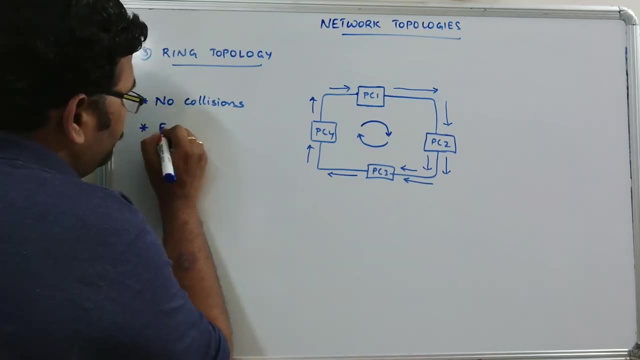 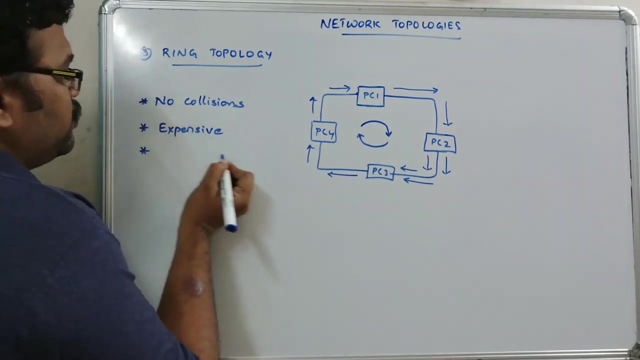 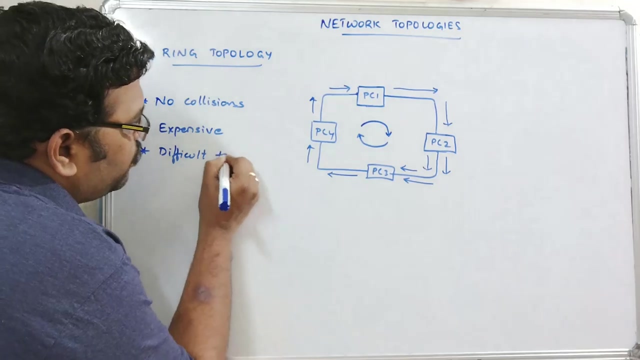 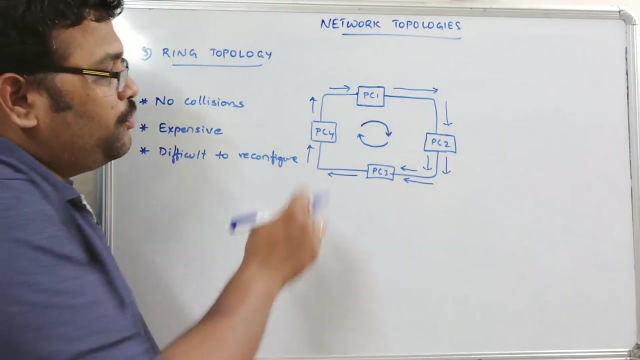 unidirectional right. no collisions will be occurred here and also the main drawback for this one is expensive, so using of more cables, and also difficult to reconfigure. that means if you want to add a more number of systems, so we have to disconnect this one and we have to correct. 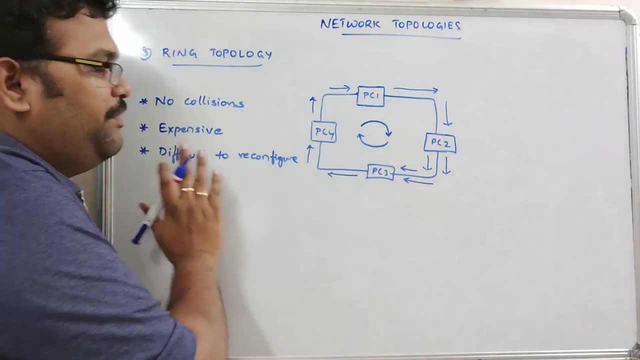 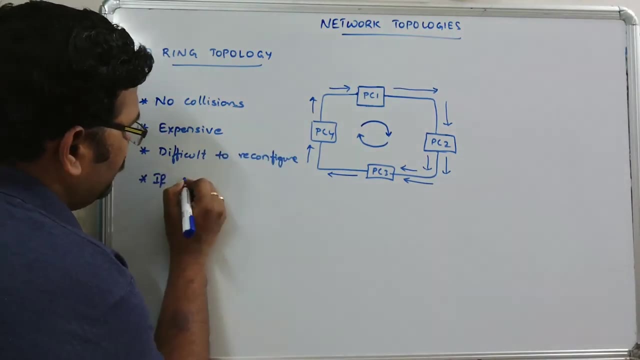 two adjacent nodes again. so that means somewhat difficult to reconfigure or expensive to reconfigure and if if you want to add more systems, then you have to add more systems, so you have to add more data to actually get decision here right, and so any system fails, transmission fails, if any. 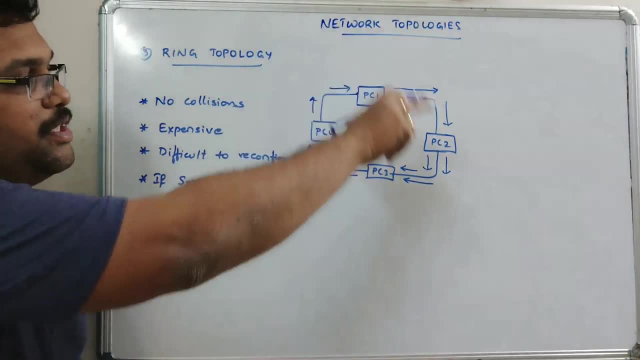 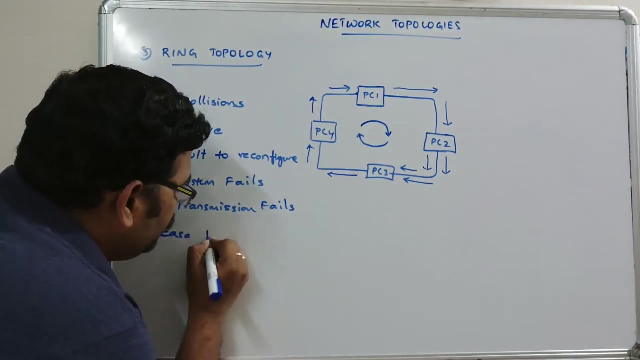 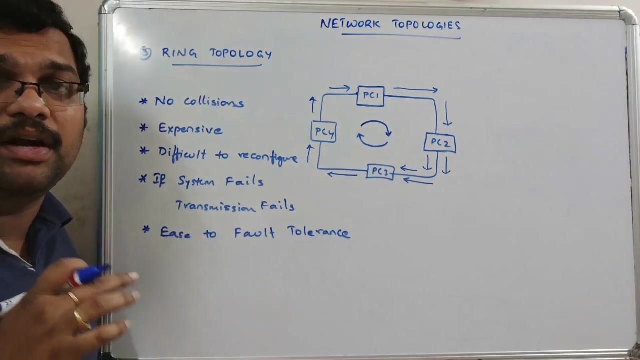 system fails automatically, the transmission will also get fail, because it is data is transmitting only with only one direction. and again, easy to fault tolerance. easy to fault tolerance. fault tolerance means identity, fault tolerance means it editor. here it is identifying the fault. so if one system gets disconnected, so it is easy to identify where. 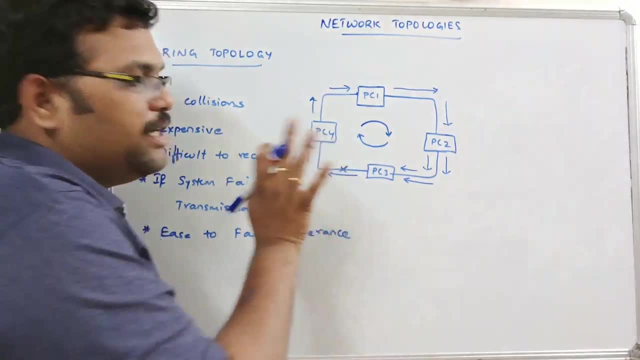 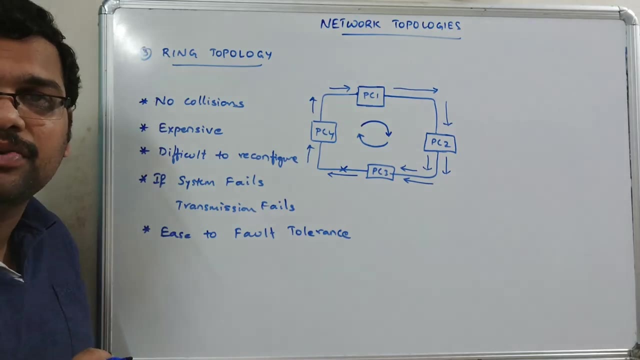 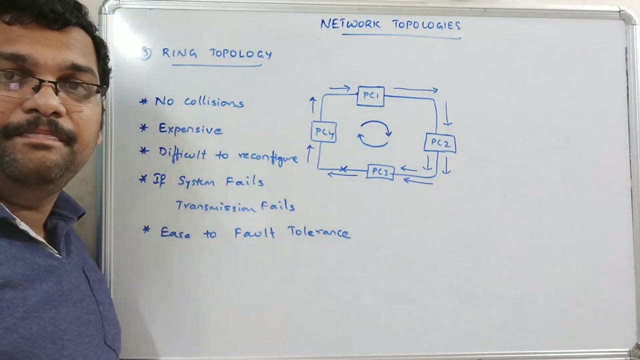 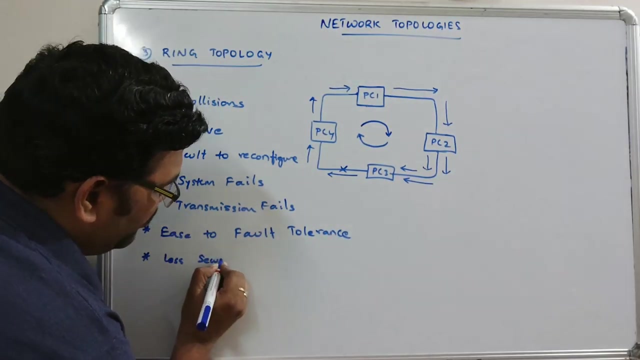 the fault occurs because, compulsory, the adjacent nodes will be get disconnected, because only two nodes will be connecting to each and every computer. so that's why it's very easy to find out the fault where actually the transmission has been discontinued, right so. and also here, less security, because the data will be passed through all the systems, right so. that's why. 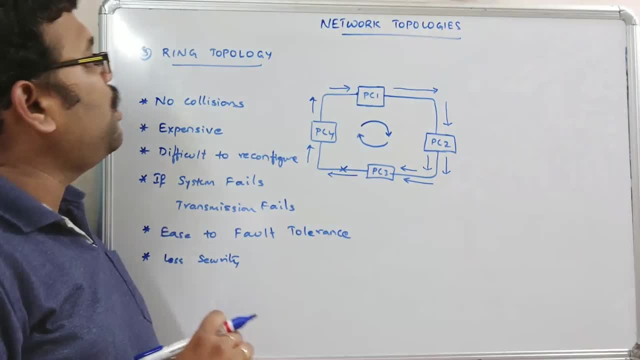 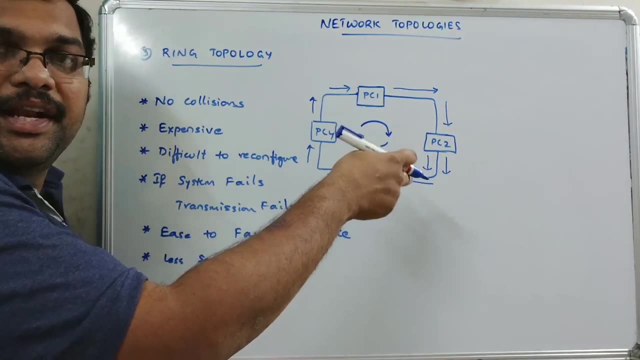 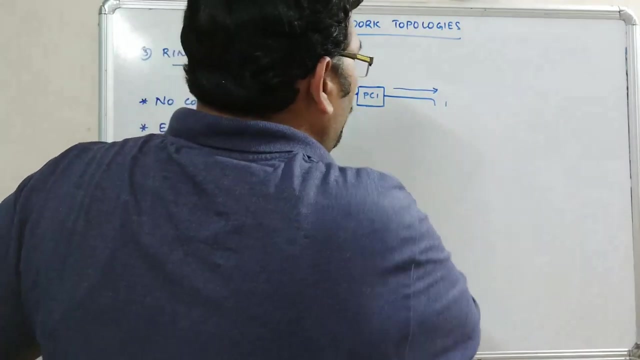 the less security here. okay, so this is all about the ring topology, because the data transmission is in the form of ring. okay, unidirectional, unidirectional, right. so this is all about our ring topology. next we will move with the another topology called mesh topology. okay, 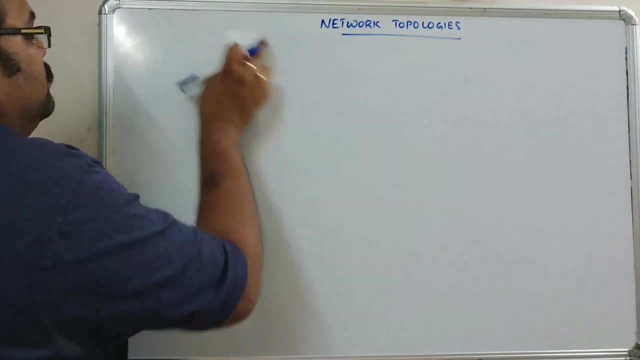 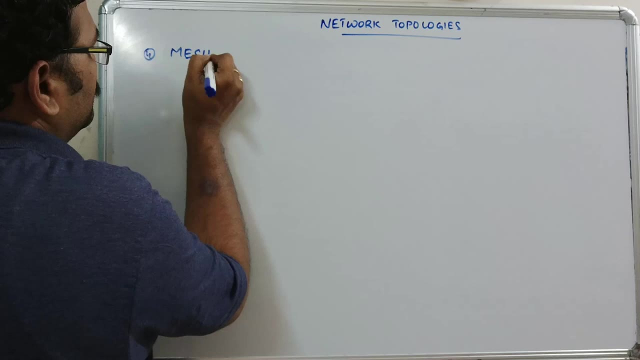 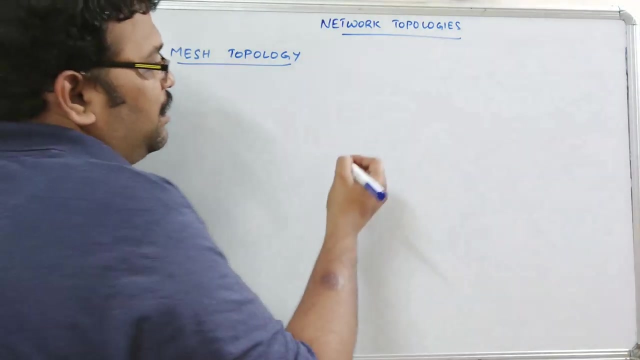 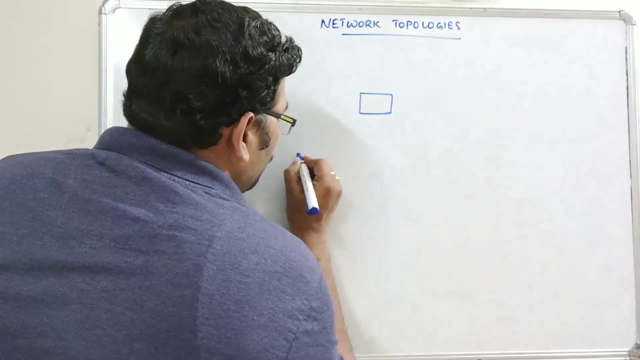 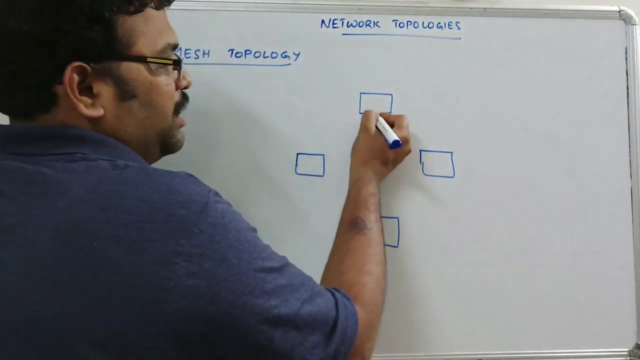 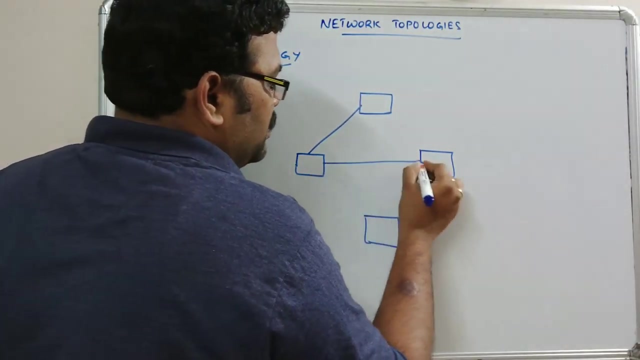 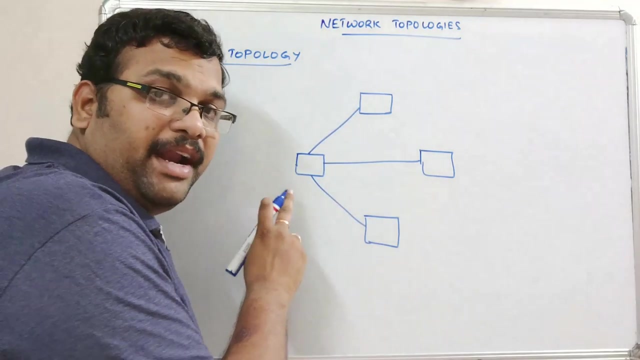 so see mesh topology. so here the mesh topology means every system is connected to all the other systems. see, for example, we will consider four systems, as we have considered in the ring topology. see, so there will be okay connection to all the three systems. and similarly, see, this is also a bidirectional, this is a 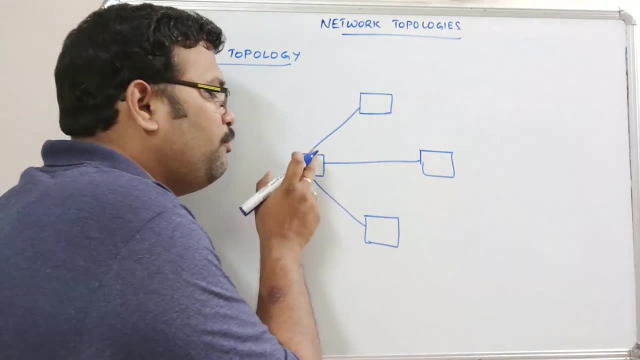 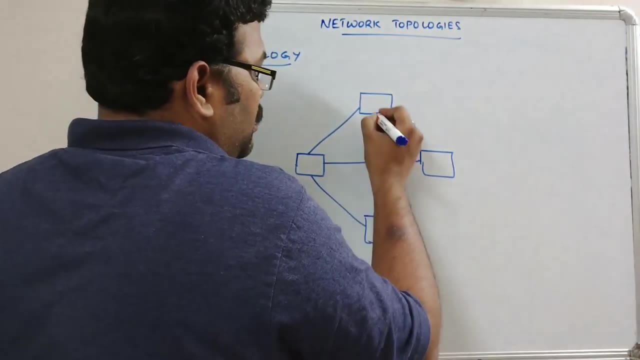 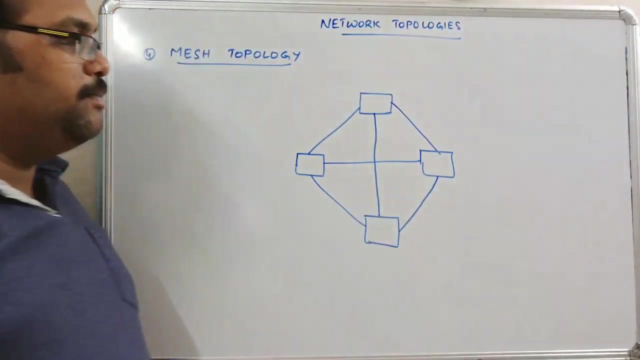 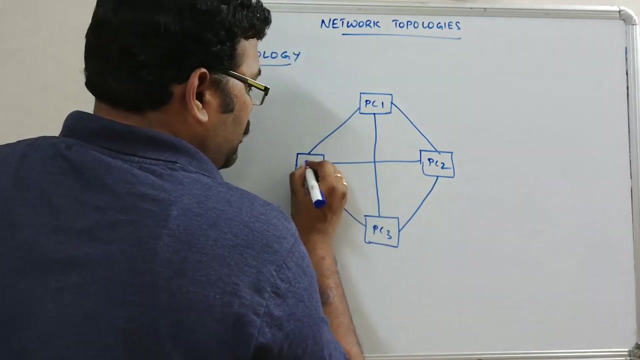 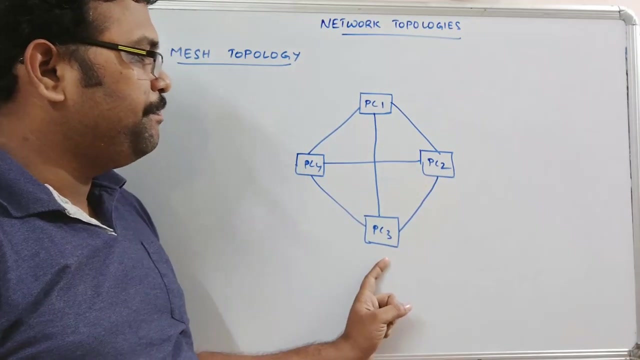 bidirectional. bidirectional means data can be sent from one computer to, i mean this computer to this computer and as well as this computer to this computer. so right, so you can observe here: PC1, PC2, PC3, PC4. see PC1 is connected with PC4, PC2, PC3. so three nodes, connection of three nodes. if you consider PC2, it is connected with PC1, PC4 and PC3. if you consider PC3, it is connected with PC4, PC2 and PC1, and if you consider PC4, it is connected to PC1, 2 and 3. so this is the client service. 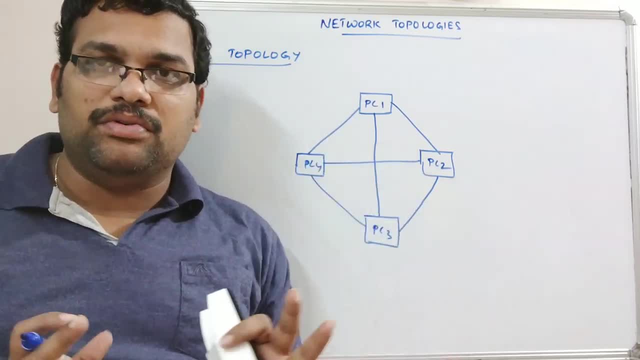 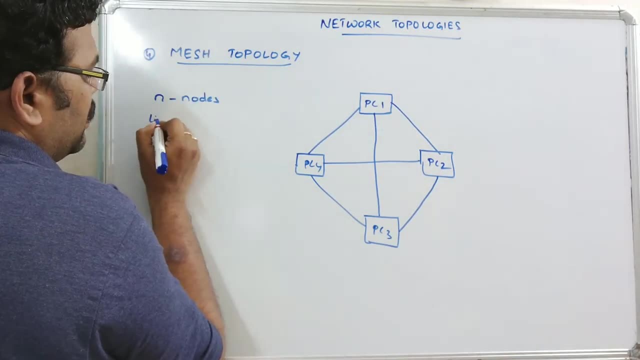 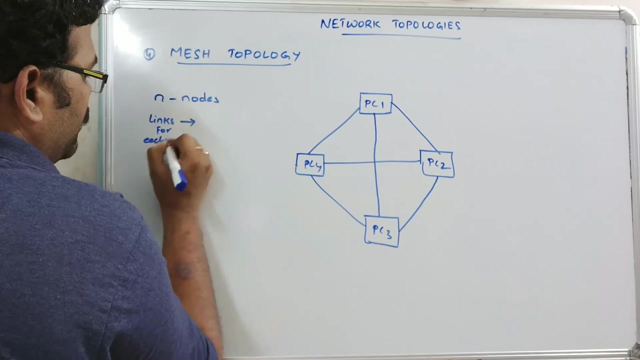 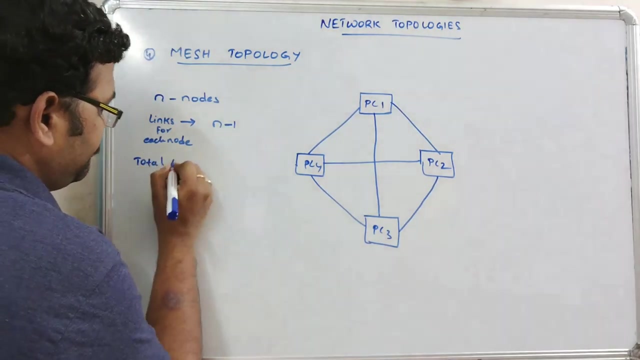 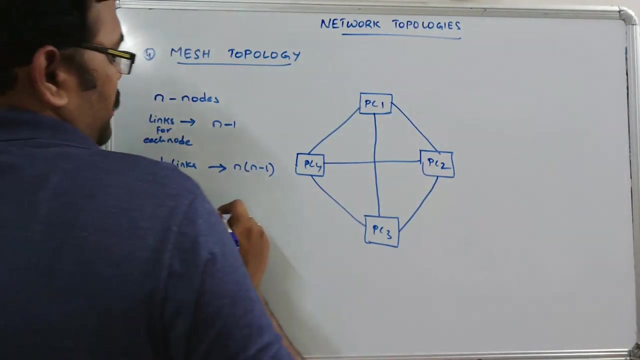 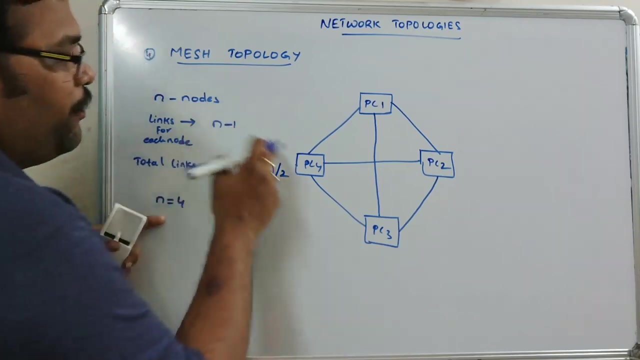 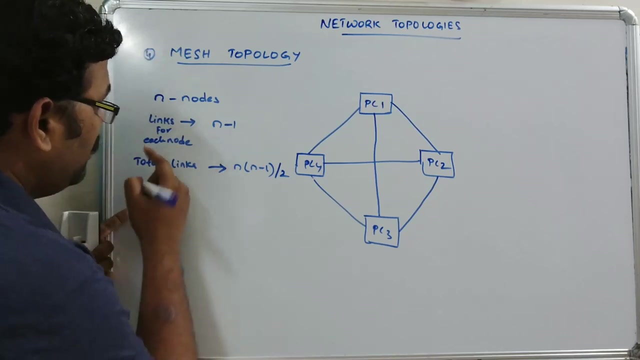 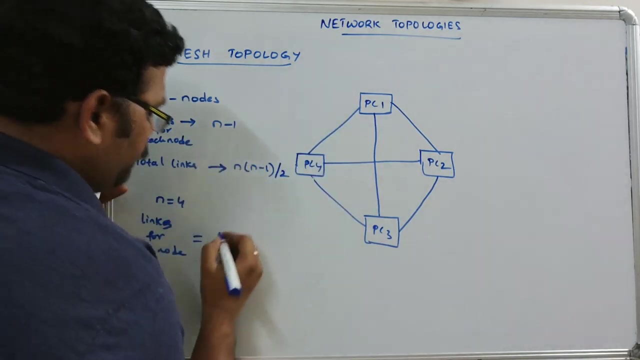 So each and every node is connected with all the remaining nodes. That means if there are n nodes in a network, so links for each node will be n minus 1 and total links will be n into n minus 1.. See, you can observe here. So here there are 4 nodes. It's a bidirectional, n is equal to 4.. That means 4 nodes: 1,, 2,, 3, 4.. Next, links for each node: Links for each node will be n minus 1.. 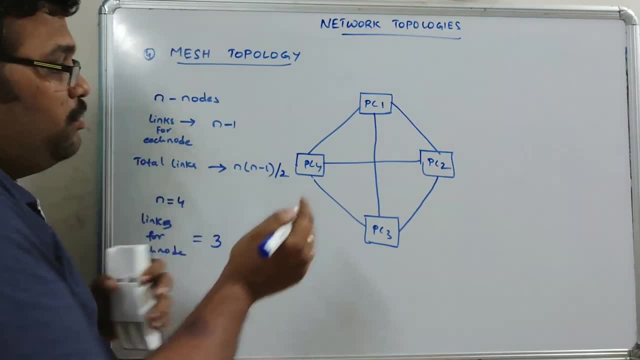 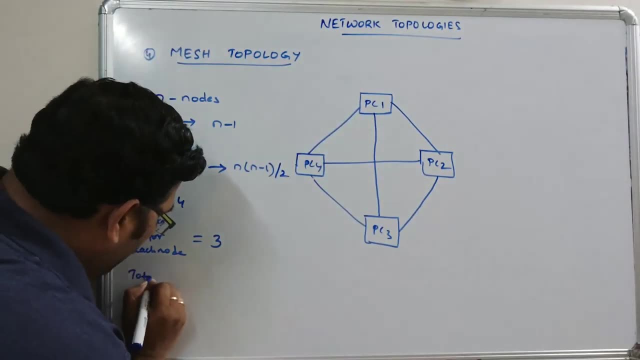 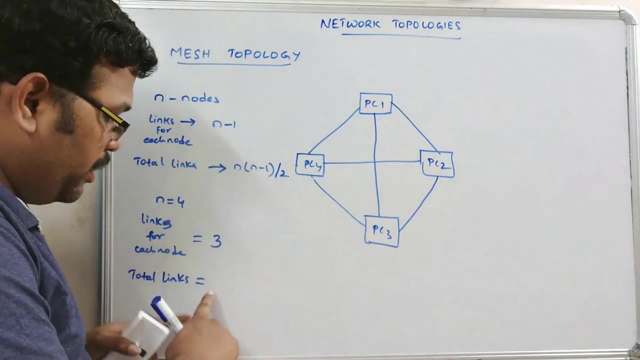 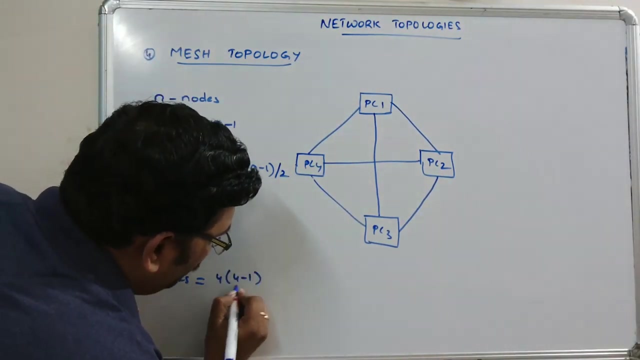 That means 3.. That means 1 node is connected to all the remaining. So see, if you consider this one, how many links are there: 1,, 2, 3.. So 3 nodes Now total links. Total links: If it is a bidirectional, the links are: n into n minus 1 by 2. That means 4 into 4 minus 1 divided by 2. That means 12 by 2, which is nothing but 6.. 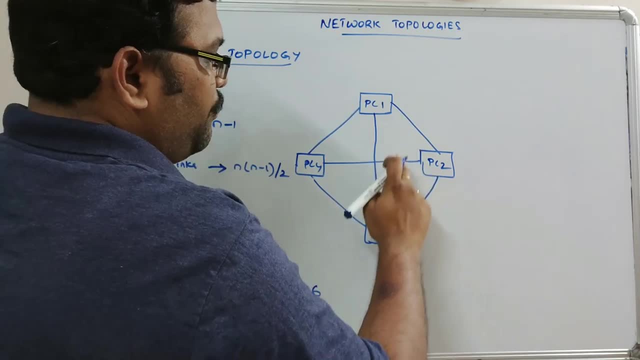 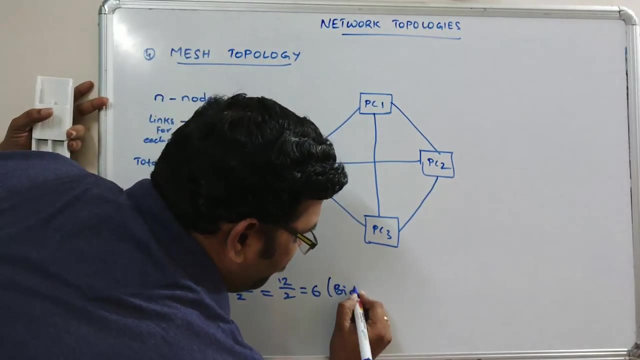 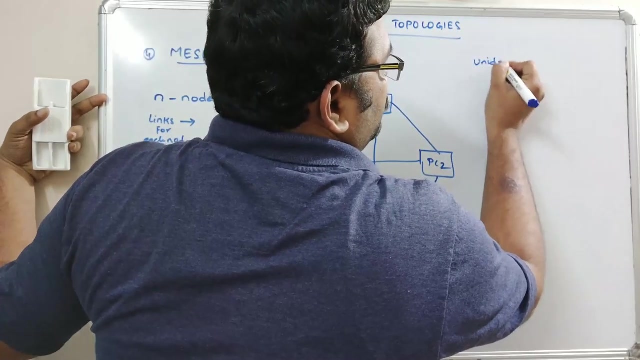 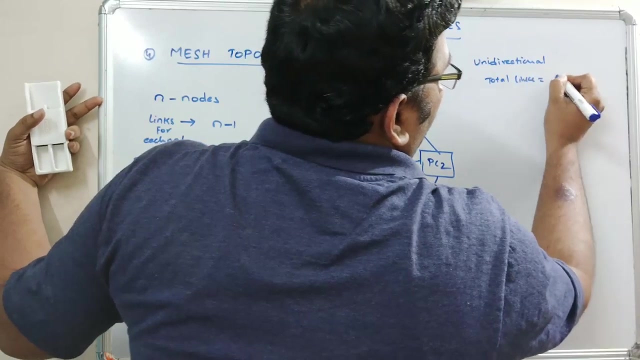 Now here: 1,, 2,, 3,, 4,, 5 and 6.. Total 6 links are available, And so this is a bidirectional, Bidirectional. If it is a unidirectional, unidirectional, total links will be n into n minus 1.. 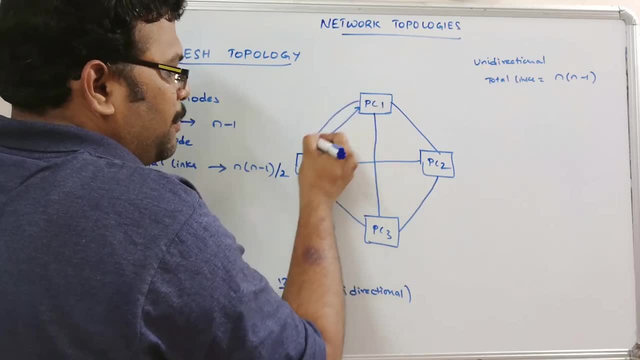 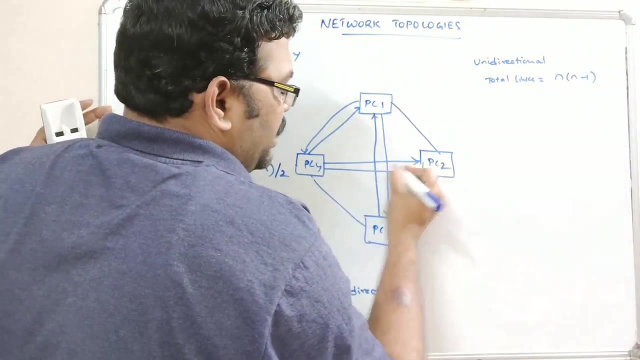 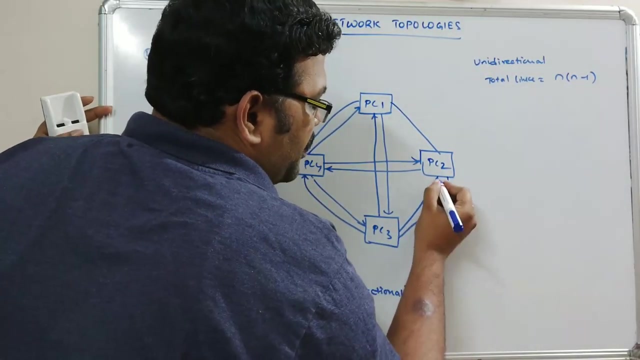 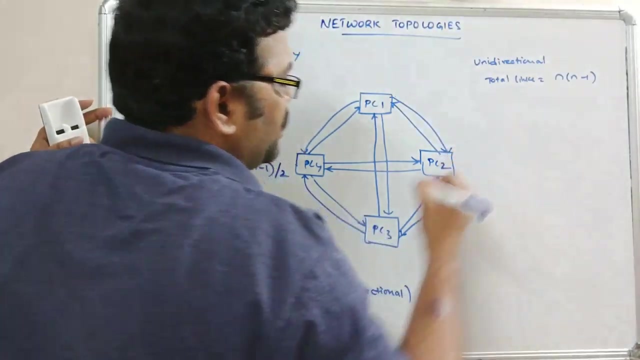 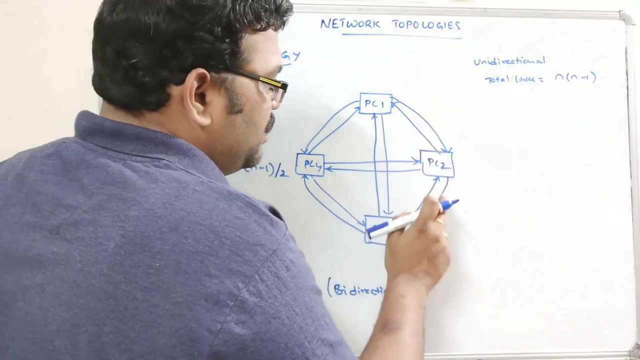 That means see Sending, Receiving, Sending and receiving, So you can observe If it is a unidirectional. So these are the nodes 1, 2, 3, 4, 5,, 6,, 7,, 8,, 9, 10.. 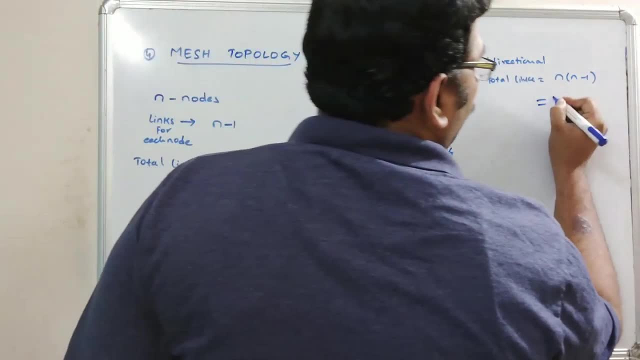 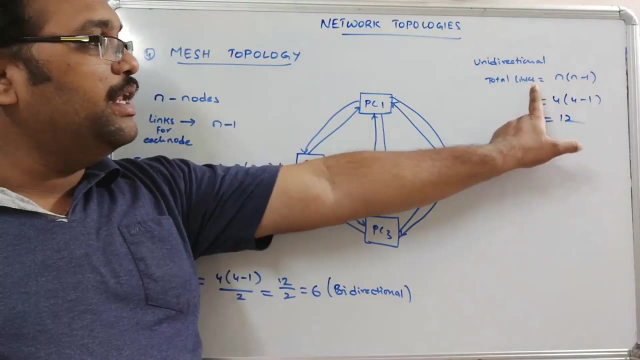 And 11 and 12.. So total 12.. So here you can observe 4 into 4 minus 1, which is nothing but 12. So if it is a unidirectional, the total links are 12.. If it is a bidirectional, the links are n into n minus 1 divided by 2. That means 6 links. 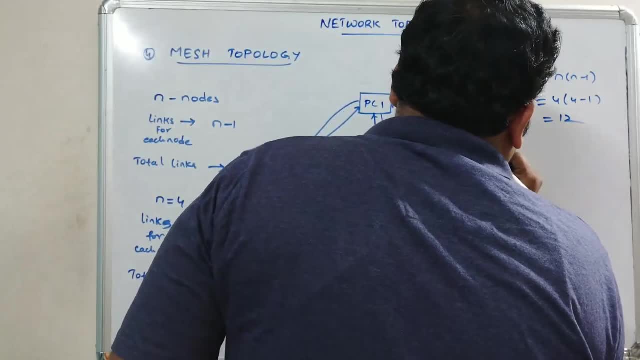 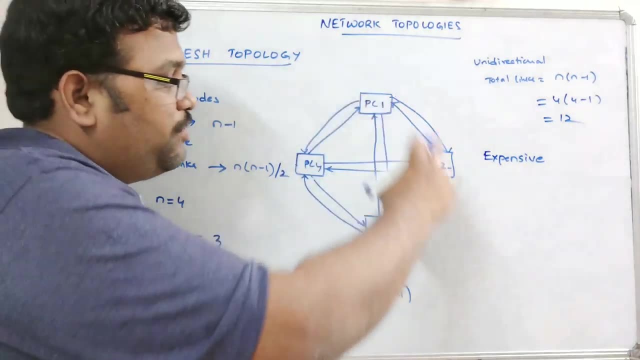 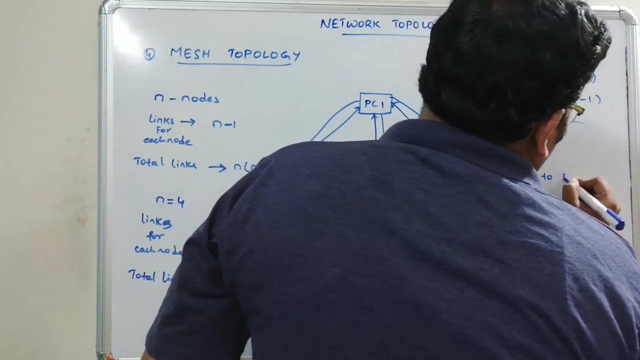 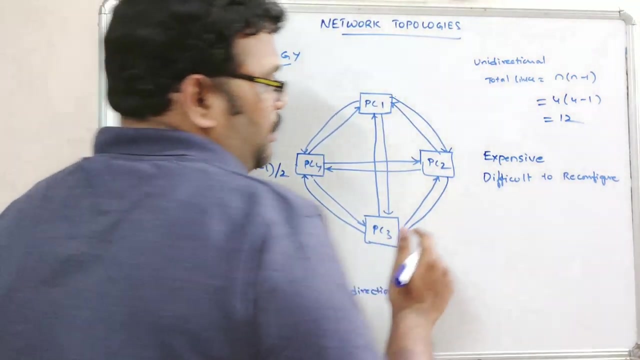 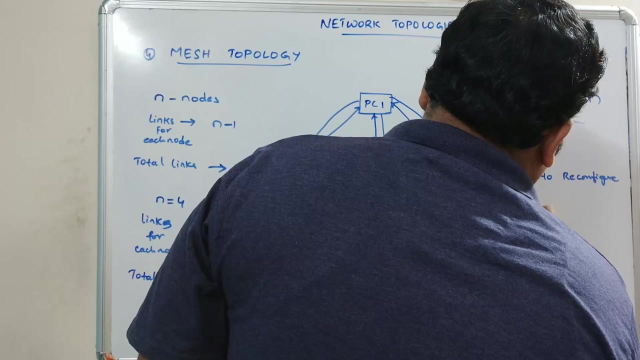 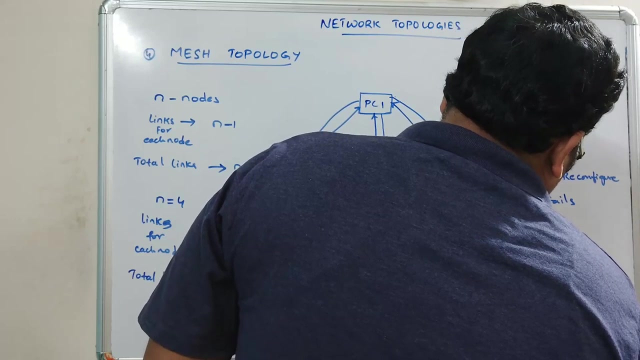 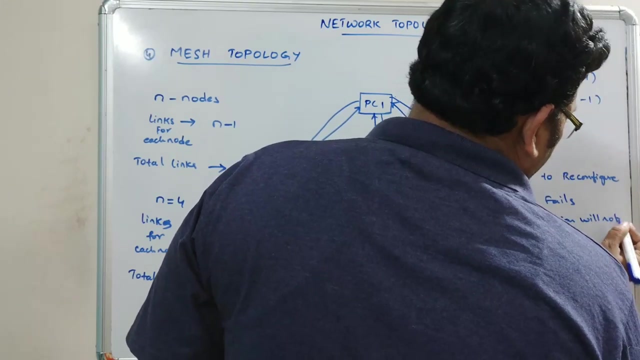 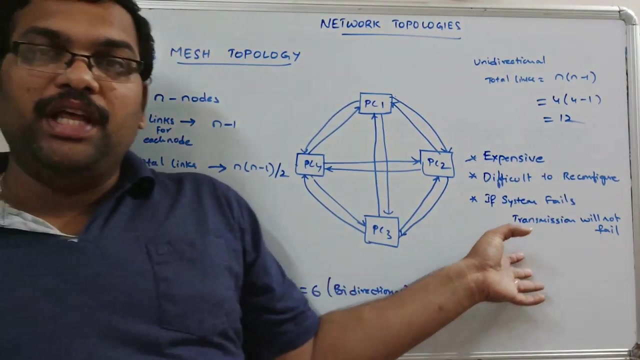 So here also it is expensive, Expensive because lots of cable will be available, And difficult to reconfigure. So adding and deletion of systems is difficult And if any system fails, Transmission will not fail. If any one system fails, the transmission will not fail, It will move with an alternate path. 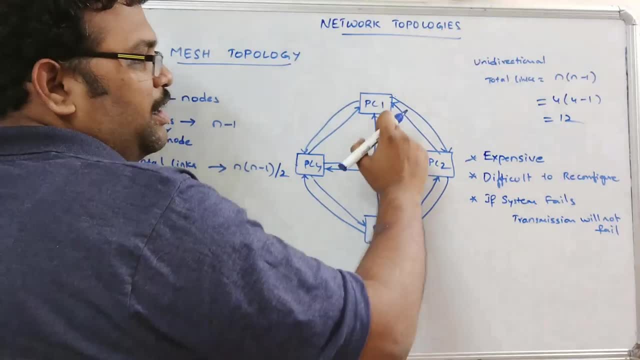 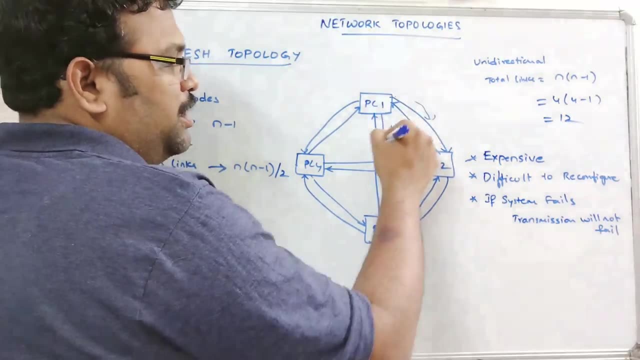 So if PC1 wants to communicate with PC3, if the data is sending from in this way, if PC2 fails, automatically that will be moving in this way. So there are some alternates, because every system is connected with all the remaining systems. 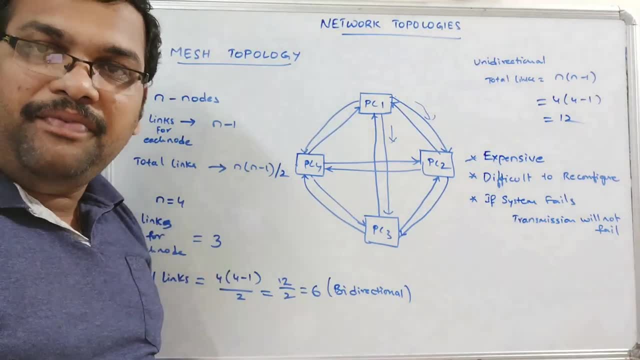 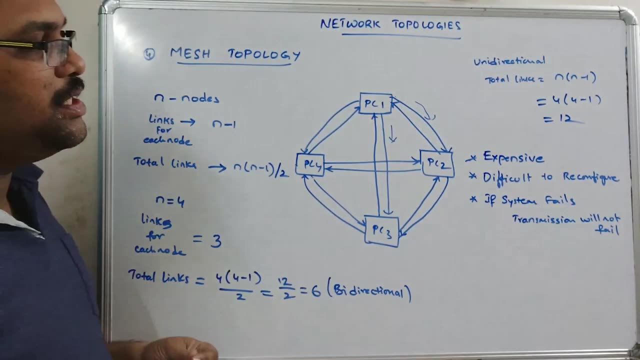 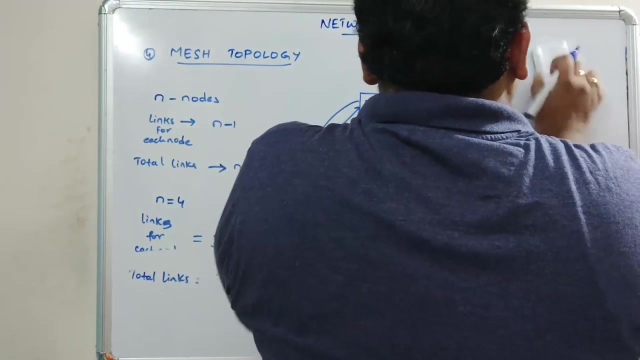 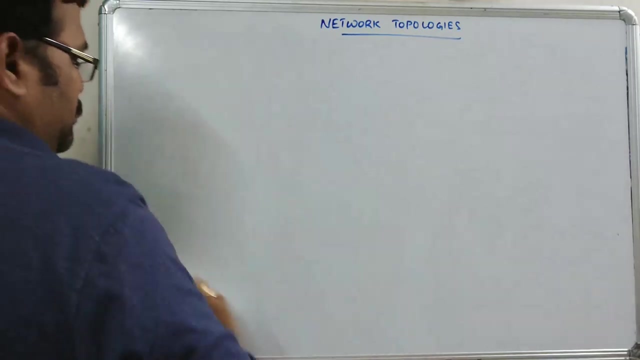 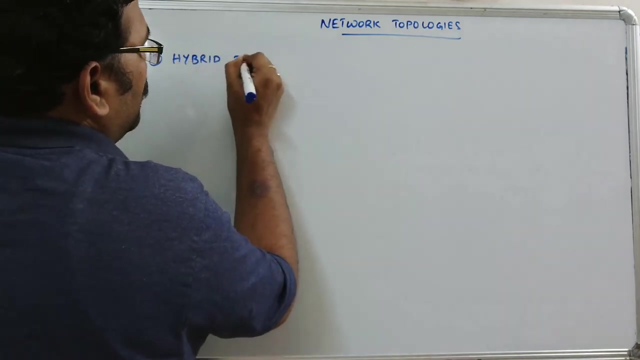 So that is. That is why if system fails, the transmission will not get affected in this mesh topology, Right? So hope you understood this. topologies- And there is one more thing that is a hybrid topology. So hybrid topology is nothing but a connection of two or more topologies. 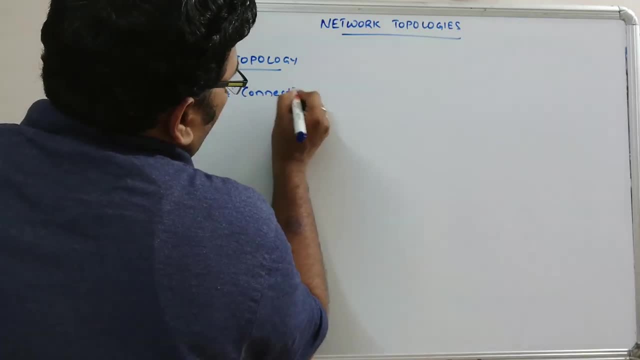 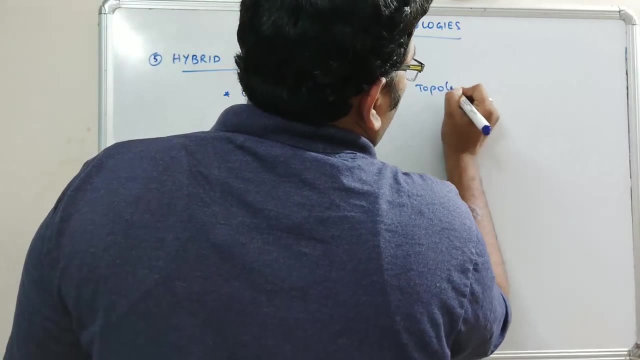 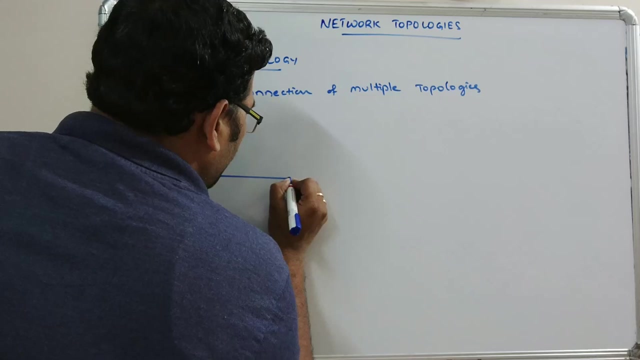 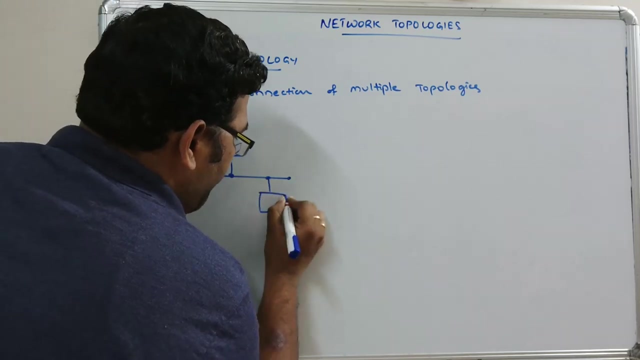 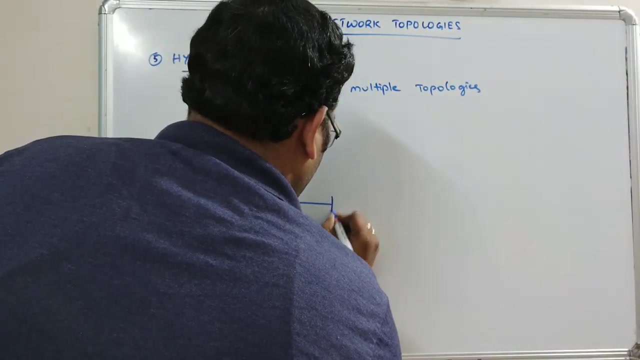 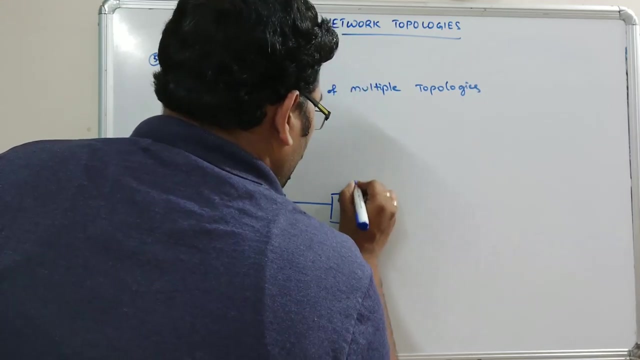 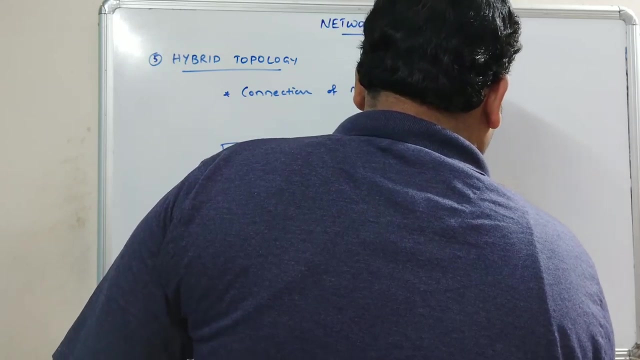 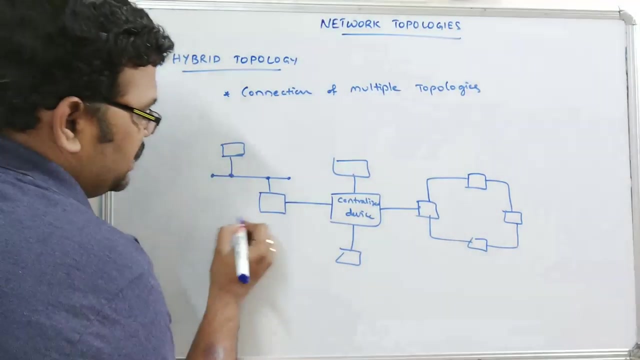 So connecting connection of multiple topologies is called a hybrid topology. For example, if you consider the mesh, the bus topology, See if you consider this one, So this is So, this is So. this is called a bus topology. 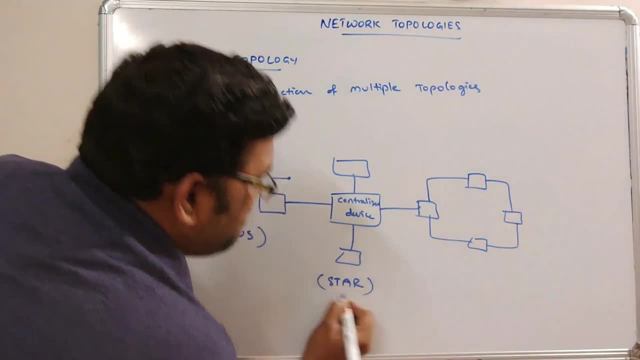 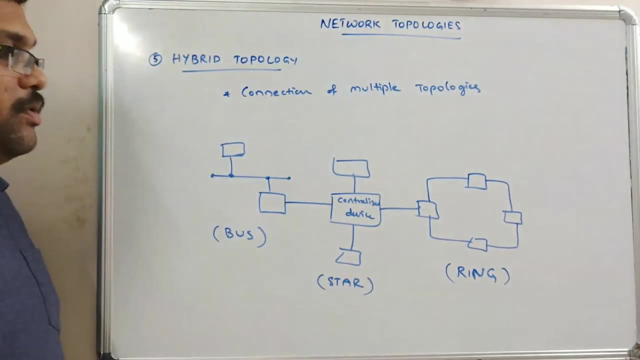 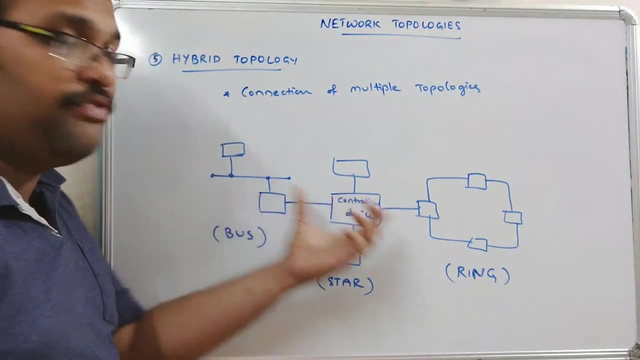 This is a star topology. This is a ring topology, Ring topology- So this connection of multiple topologies, we call it as a hybrid topology. It is also very expensive because a lot of cable will be required And also it is also difficult to configure because of adding more number of systems. 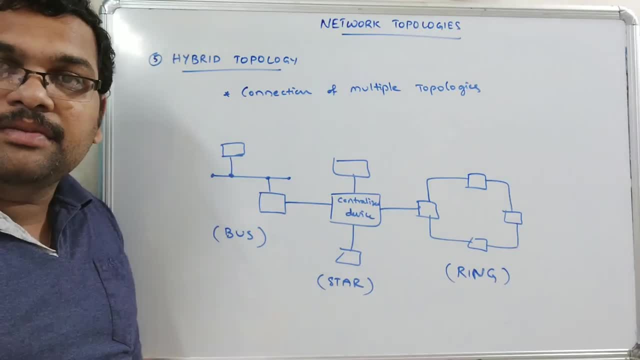 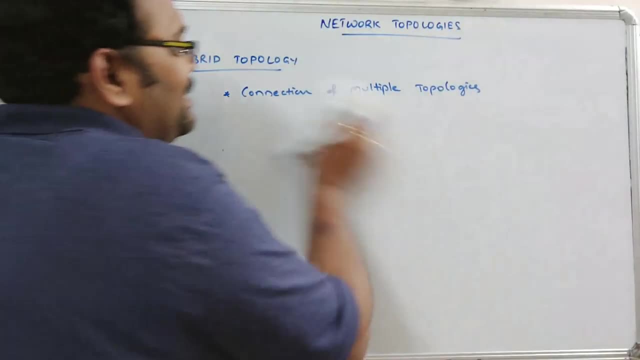 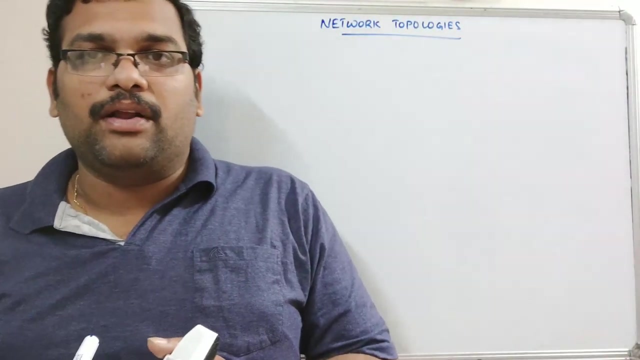 Right. So this is called a hybrid topologies, Right? So hope you understood, guys. So mainly the topology means arranging the computers in a network. So how many ways we can arrange these computers in a network, to connect a network.